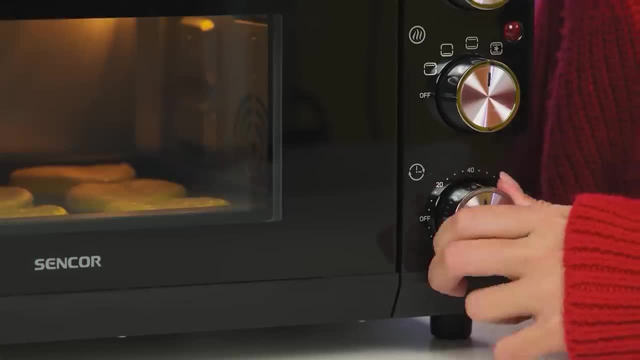 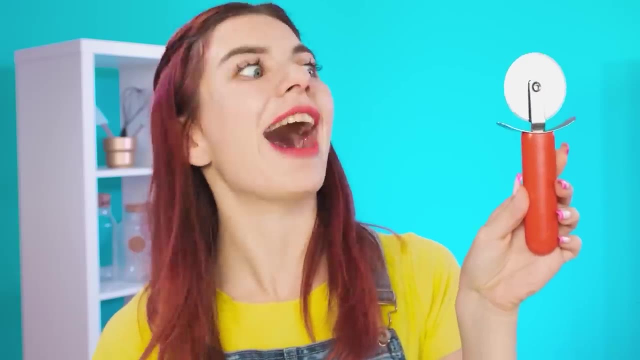 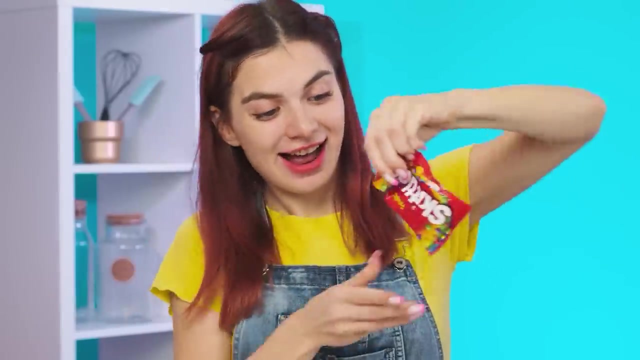 on a baking sheet. Get into the oven. future cookies: I can't do anything. Good idea: Cookies are round, right, So you can just cut a circle out of the dough and not bother. And the most important ingredient is kettles. 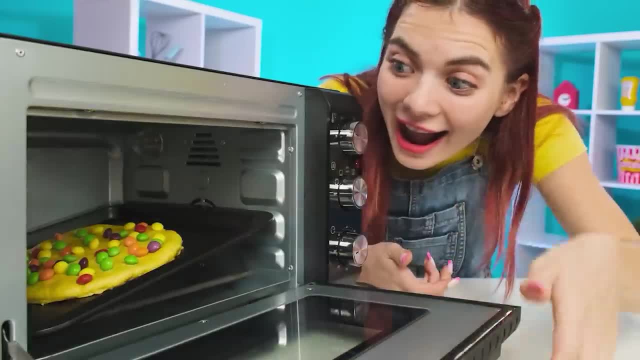 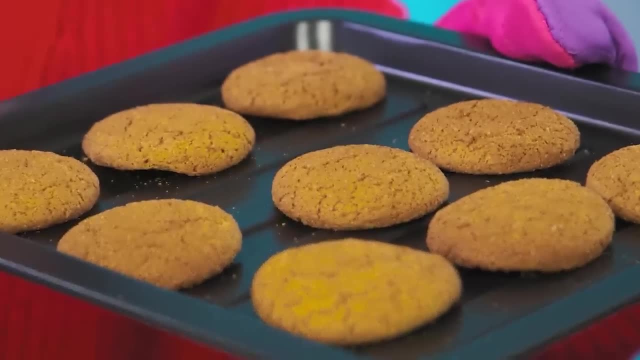 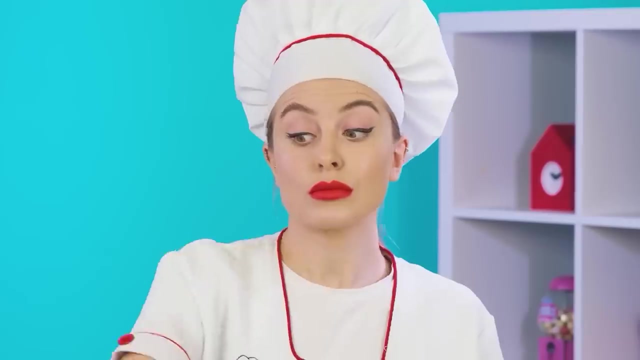 I don't mind having a snack with such cookies myself. You did a good job, honey. And how are my cookies? Without exaggeration, as always perfect. I will leave no comments. Here are my cookies. This is a work of art. 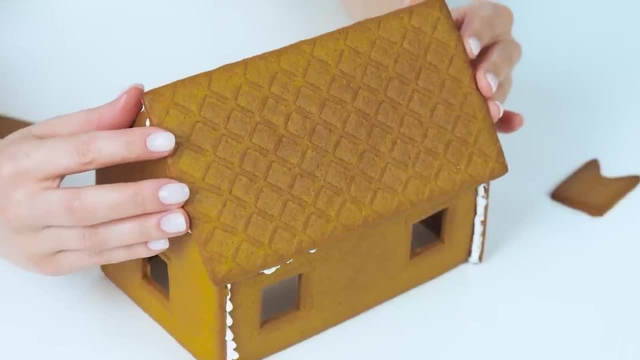 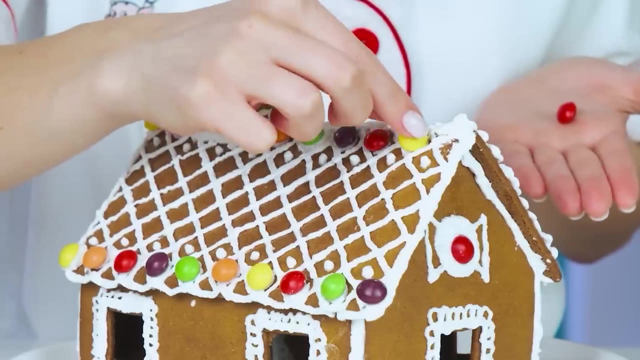 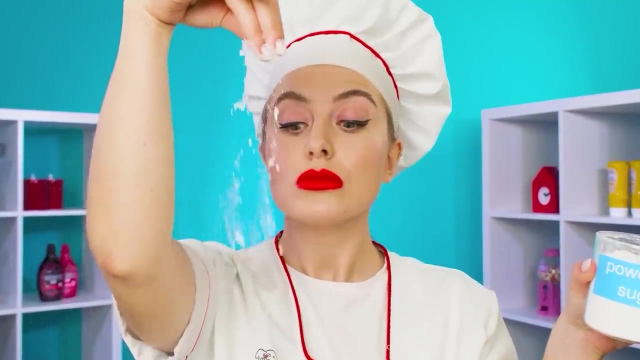 The master's hand is immediately visible. Just look at what an amazing gingerbread house I have. By the way, thanks for the idea. I'll decorate the roof with skittles. Well, the final touch, Powdered sugar, And my house seems to be dusted with a snowball. 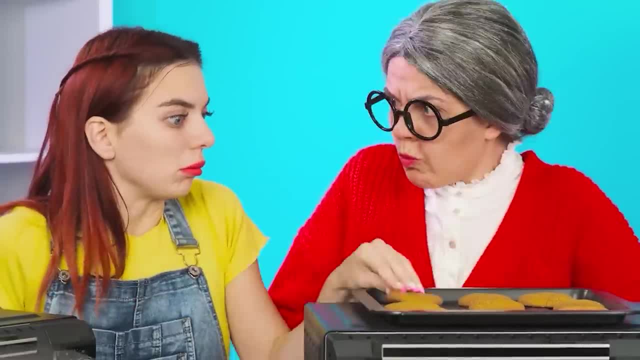 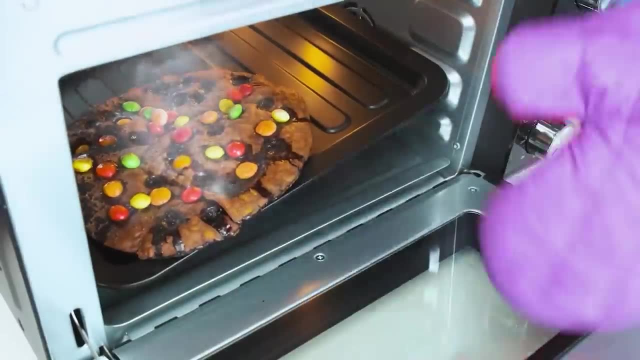 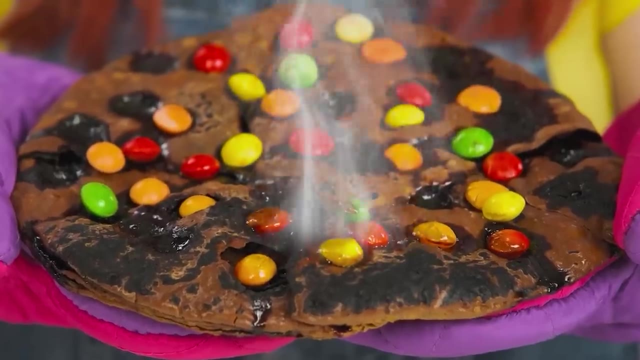 I can't believe my eyes, Darling. these are not for you. Oh no, Looks like a small fire. We need to get cookies urgently. Maybe it can still be saved. Oh no, There doesn't seem to be anything to be done here. 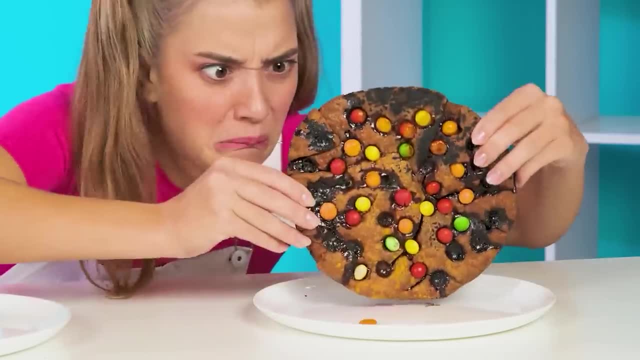 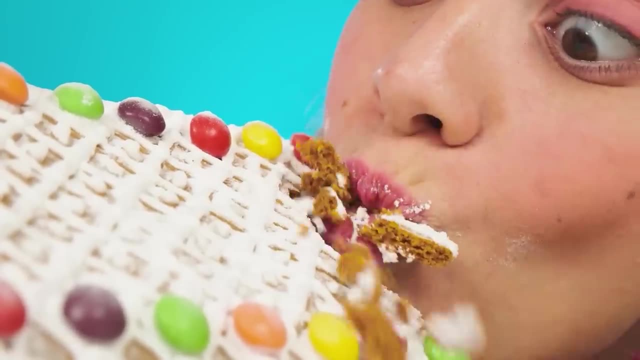 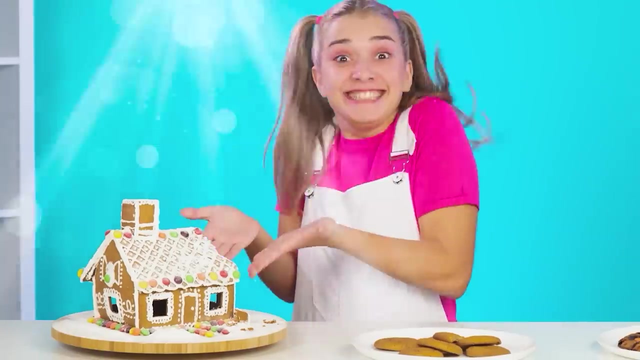 And these are cookies. I'm not sure you can eat it at all. Well, well, what do we have here? Wow, A gingerbread house, So beautiful And so delicious. Hmm… I think this house has one, And it couldn't be otherwise. 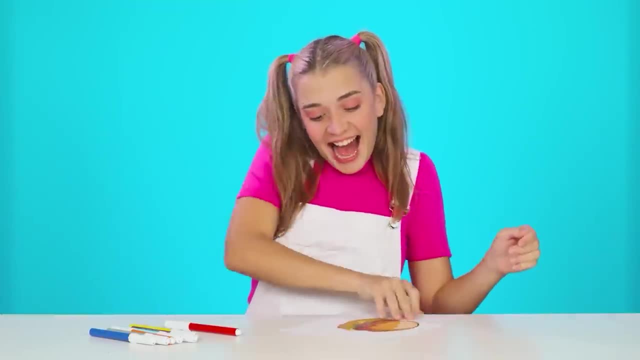 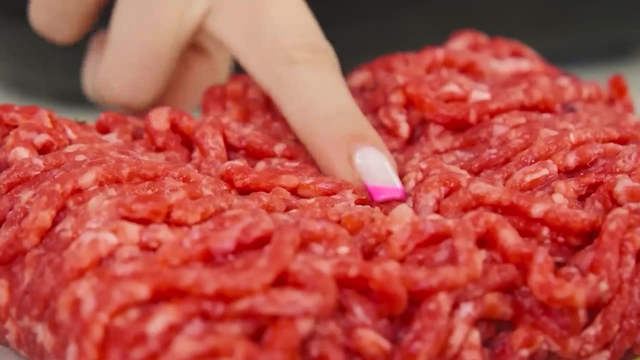 I'm a professional And now I want a burger, And quickly. I can do it, Although maybe not. Is that mincemeat? What an abomination, I know. Instead of this nasty mincemeat, you can use a…. 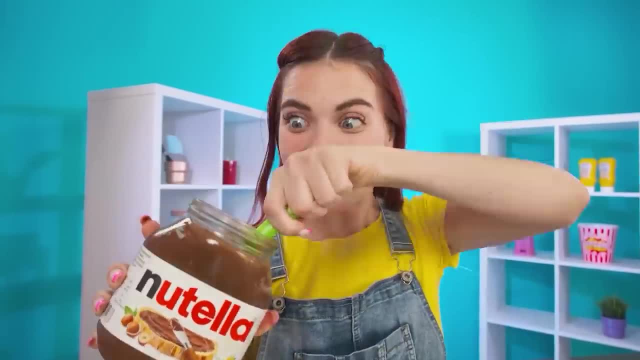 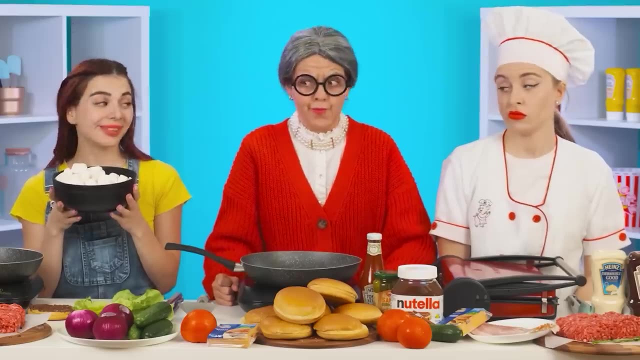 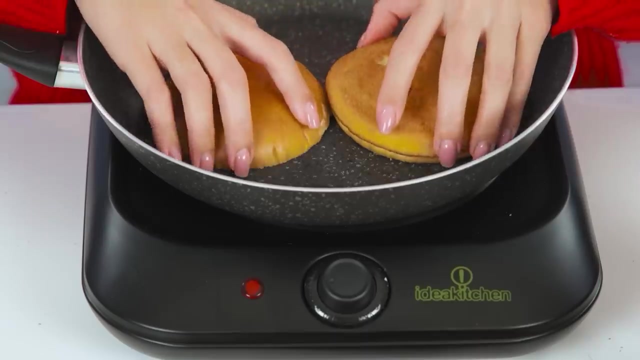 a delicious and appetizing chocolate taste. It is turning out great, Perfect. How are others doing Such perfect buns? But you need to fry them. A rubby crust will be very useful. What do you know about a rubby crust, grandma? 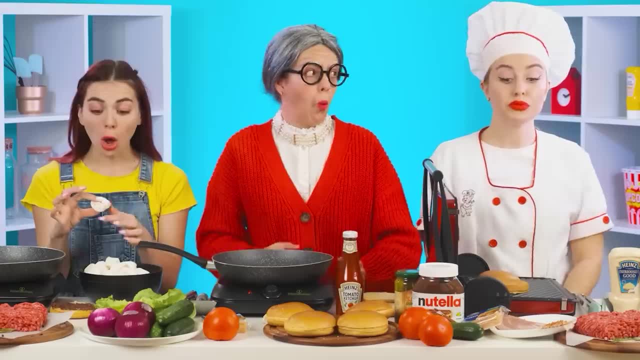 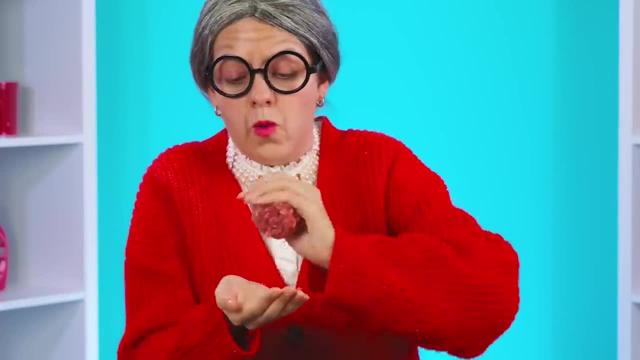 Want two and the burger is almost done. Impressive, But the most important thing in a burger is a juicy patty. I'll borrow mine's meat, thanks, And now you need to put the future patty in the pan and wait a little. 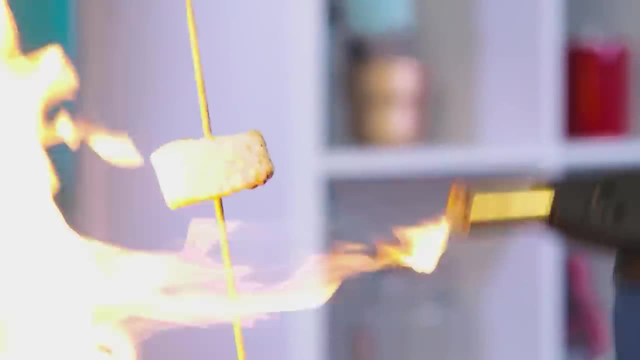 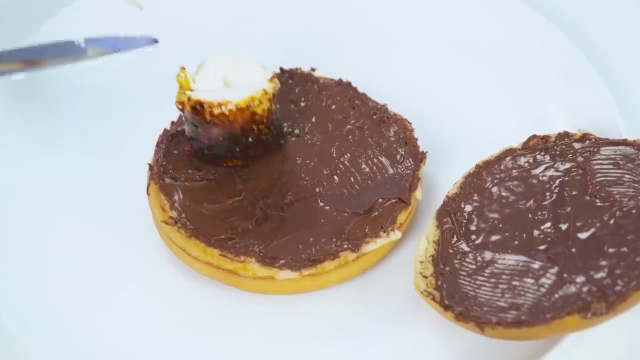 My goodness, Honey, what are you up to? Calm down, grandma. I have everything under control. I just decided to fry marshmallows and add piquancy to my burger, And now it's the turn of marmalades. 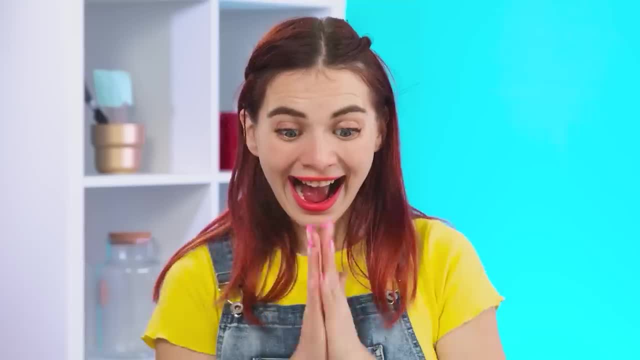 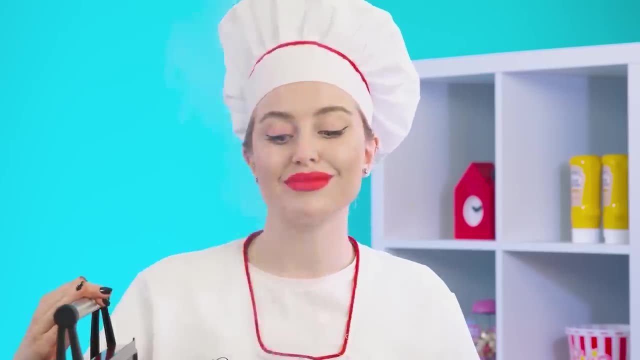 Roll on top and press harder. That's the whole recipe. How do you like it? Why this rivalry if I still make the most delicious burger? Just look at these patties. I'll add more bacon. There's never too much meat. 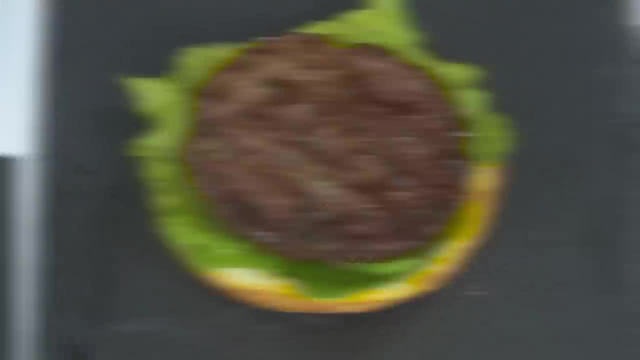 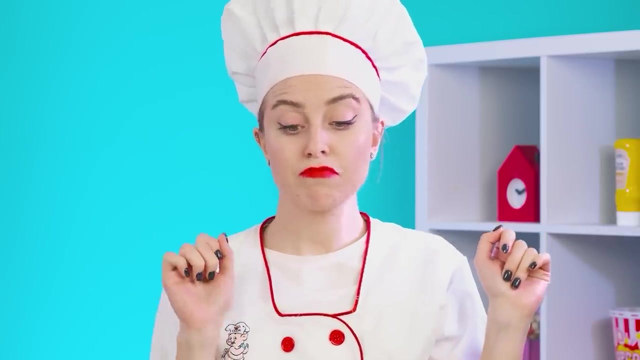 And now it remains only to lay up the vegetables and cheese in layers. I agree that one layer is very boring, But if you make a lot of layers, it'll be what you need. You just have to spread the sauce all the way. 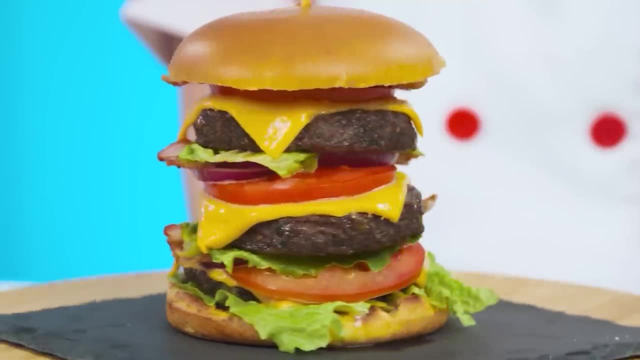 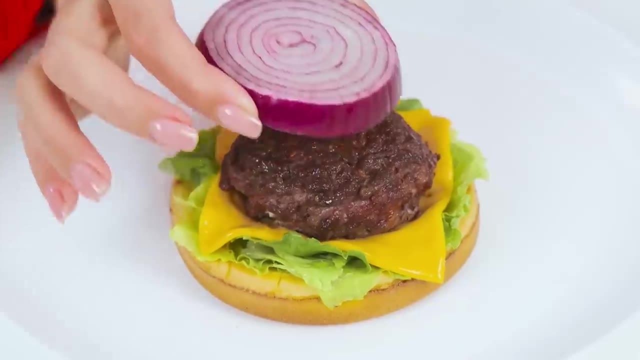 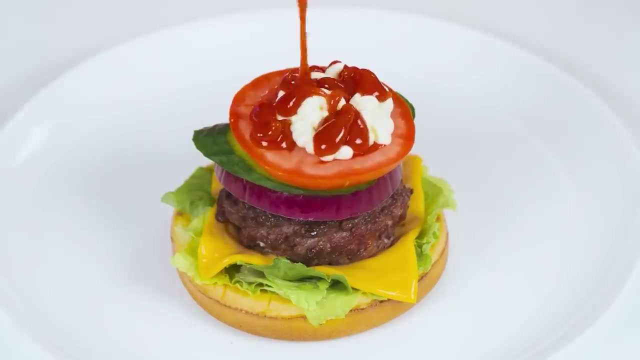 Yes, I'm a clear favorite here. It turned out absolutely great. Oh no, I'm not going to lose. Carefully lay up ingredients and now sauces. There's no need to stunt, we're doing it from the heart. What a cute burger. 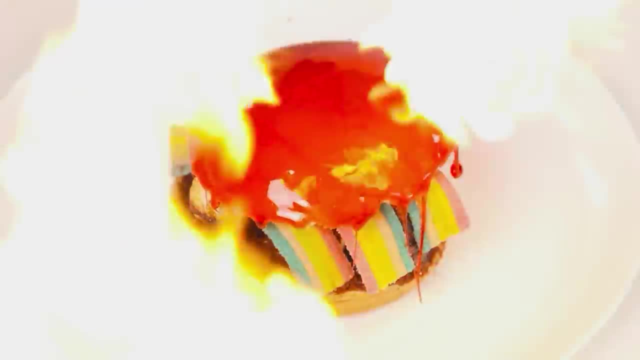 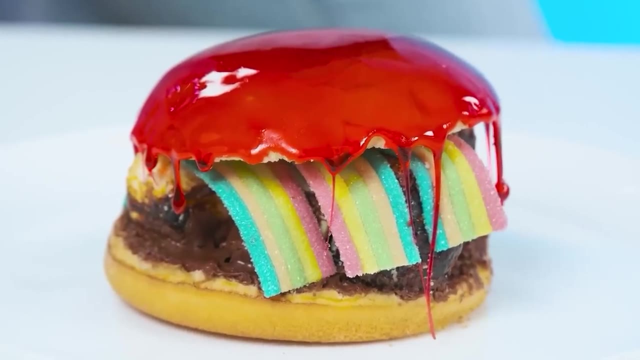 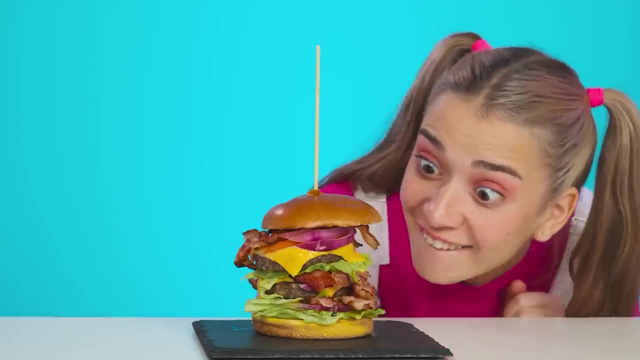 A little more and I'll achieve a golden crust. Oh dear… Something is not okay. Come on, Grandma, Look how great I did Ta-da. Wow, What's the size? A three-story burger is something I want to try fast. 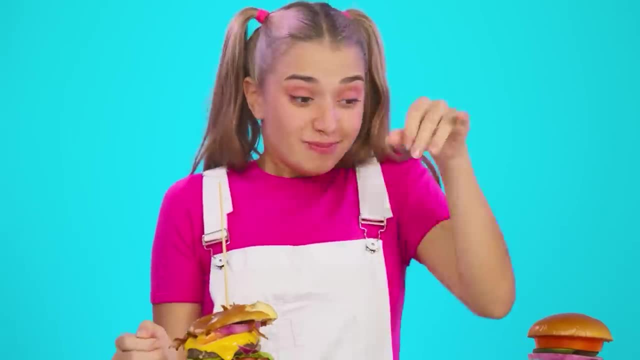 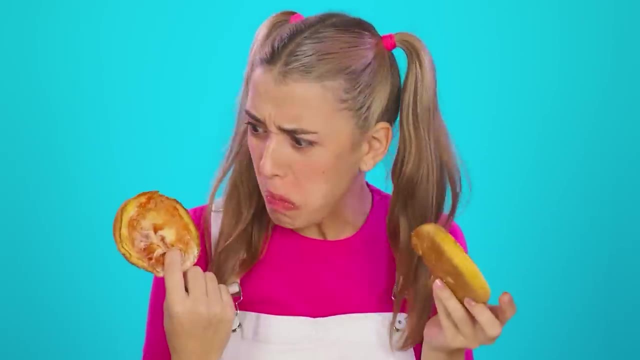 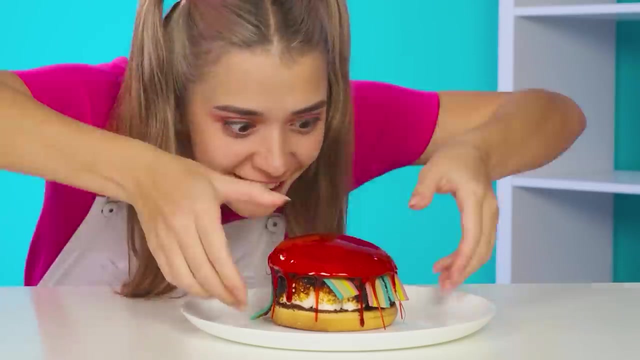 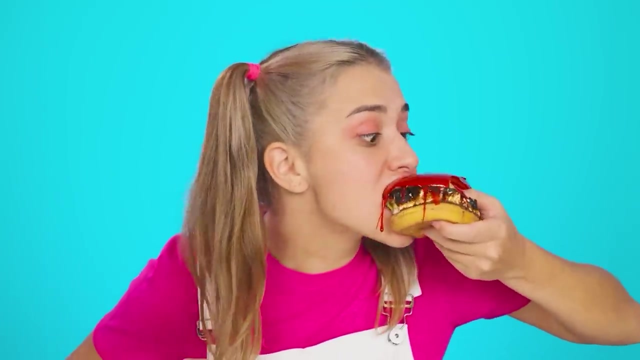 How juicy it is Amazing. Now you, my friend. Oh, Everything fell apart. Okay, because there's another burger. It looks very appetizing. Let's try, Mmm. Marmaline And Nutella Great. 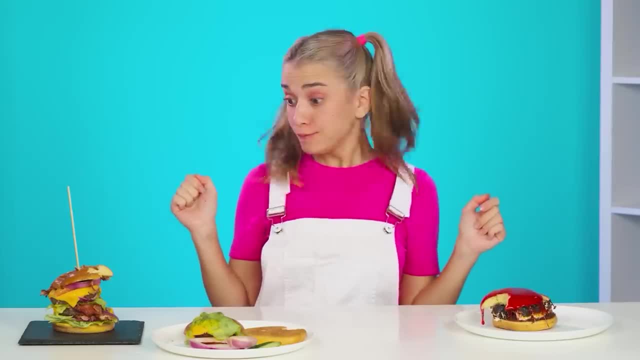 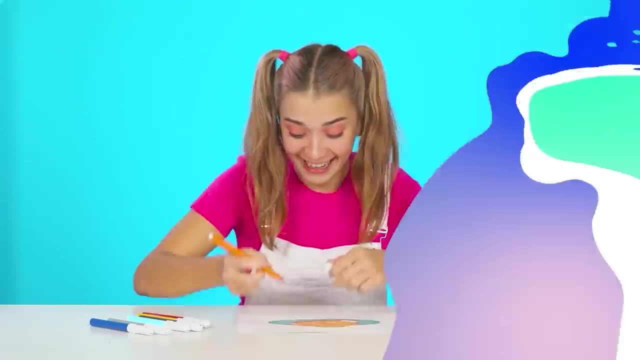 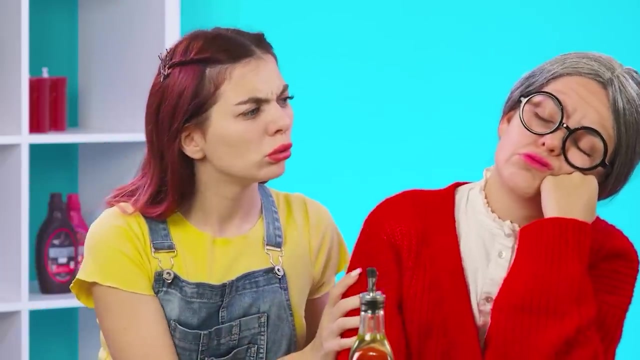 But the chef's burger wins Congratulations. Well, you know it's not fair anymore. This time I want nuggets. Will you be able to do it Easy, Grandma, wake up. Look, Jennifer wants nuggets, Okay. 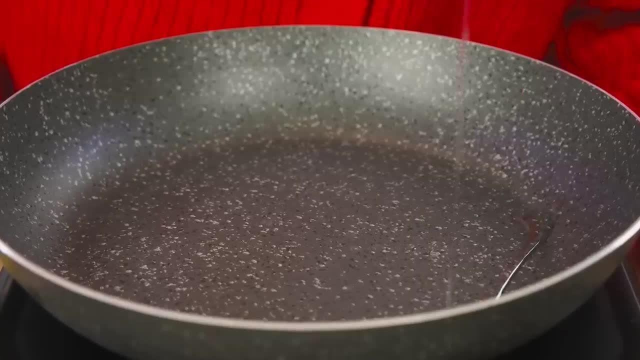 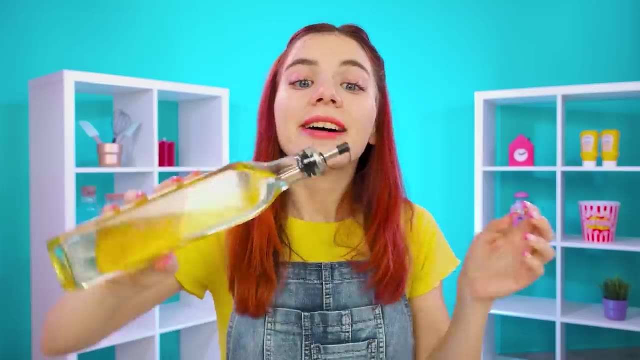 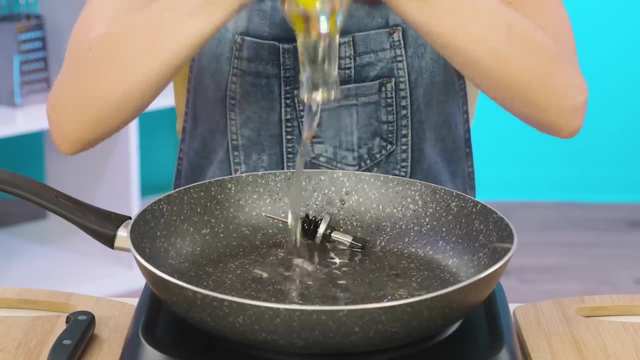 Of course. First you need to pour a little oil into the pan. Oh, Granny, will you share oil with me? Thanks, Strange, why isn't it pouring? Probably need to shake harder. Oh, come on. Oops, something clearly went wrong. 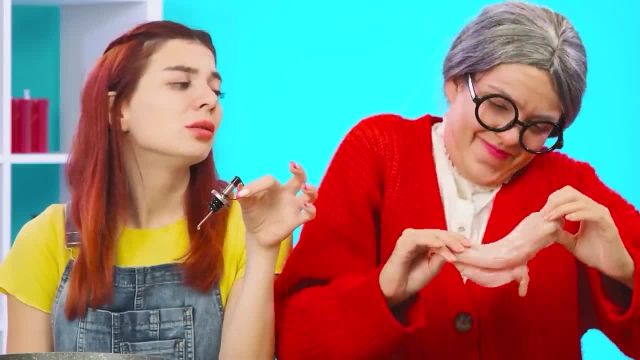 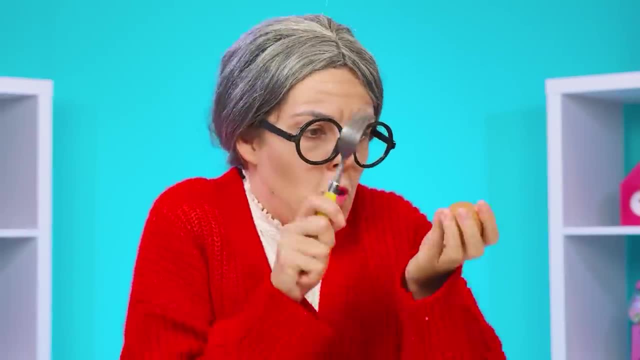 Oh dear, who doesn't like that? Okay, The main thing is that it is…. Okay, The main thing is that it is… Delicious. And to make it always delicious, I cook with love. The chicken needs to be marinated. 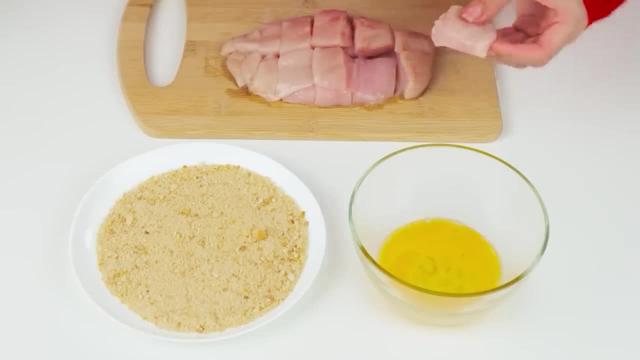 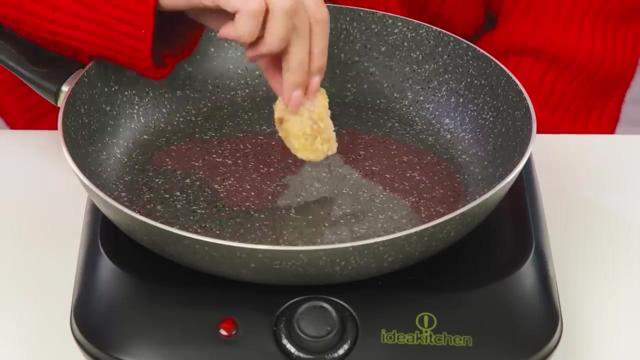 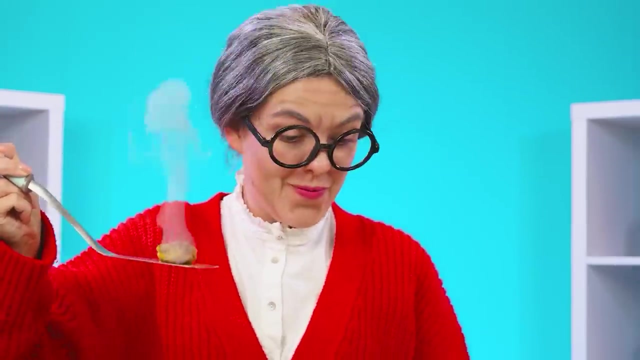 To do this: beat an egg, dip chicken pieces in it and then roll them in crackers. Great, Now you can fry it. So delicious. Yum, Barbeque, Yum. And what smell. Don't you wanna try it, chef? 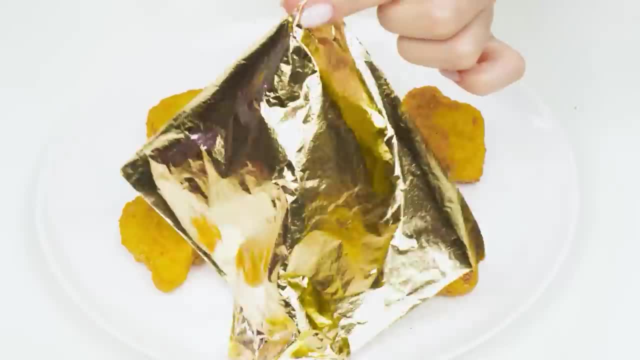 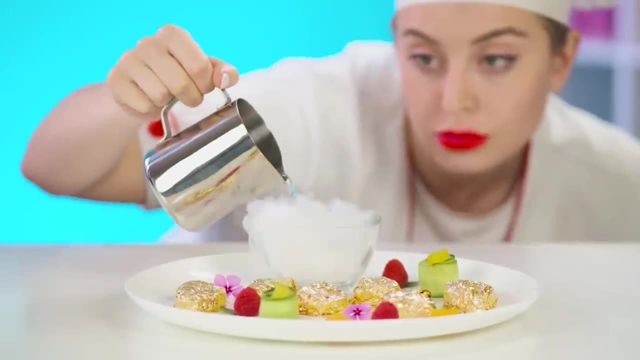 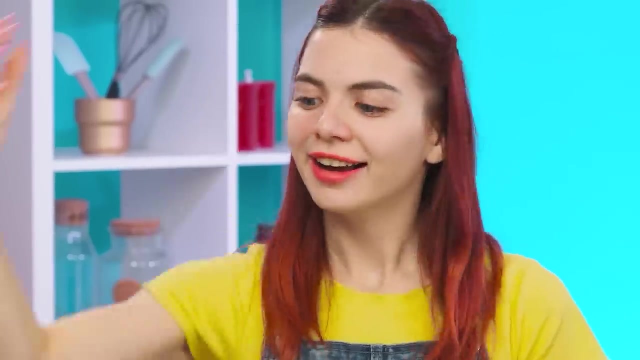 Oh no, I have something to do, something to do. My nuggets will be out of the highest class. They will look like pieces of gold And, of course, serving is also an art. It should be spectacular. I know, When you don't want to bother with cooking, you can take a pre-made one. I'll 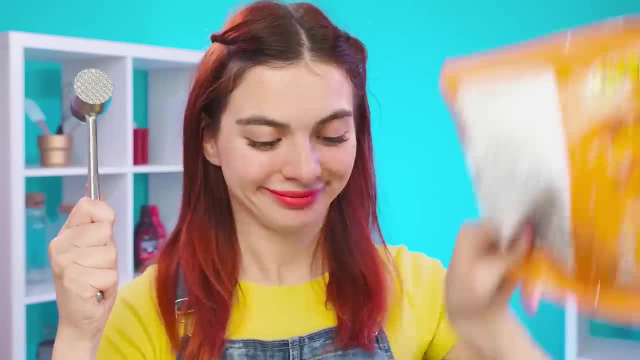 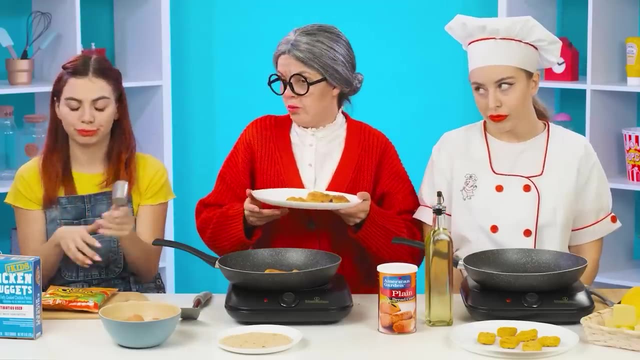 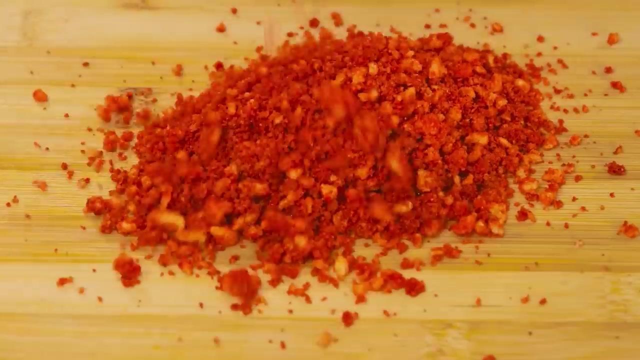 wrap the nuggets in cheese, and then I'll make the most delicious breadcrumbs from Cheetos. To do this, I'll beat this pack. well, Honey, be careful, Not so hard. Oh, It seems to have worked. We'll see. Yes, Great. Now let's add Cheetos to the 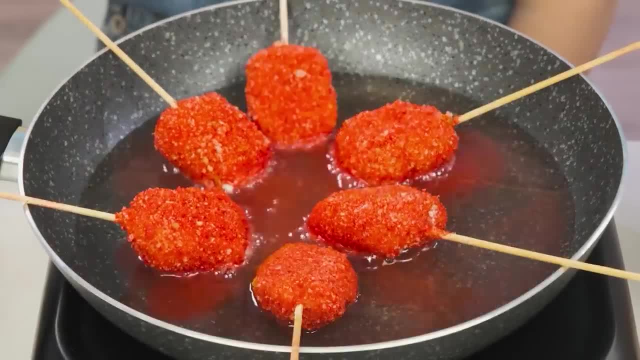 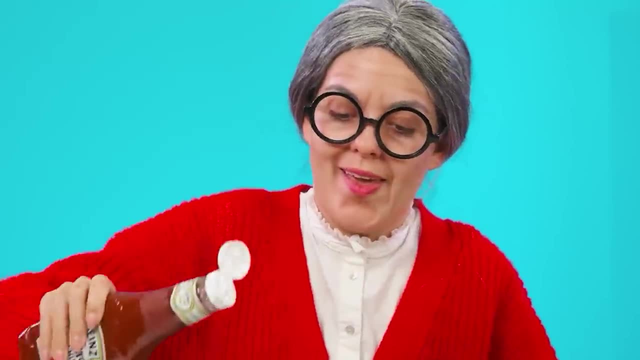 nuggets and put them in the pan. I already feel this amazing taste. Don't even want to give it to the baby. I almost forgot. Well, what kind of nuggets without ketchup? Now it is perfect, Woohoo. 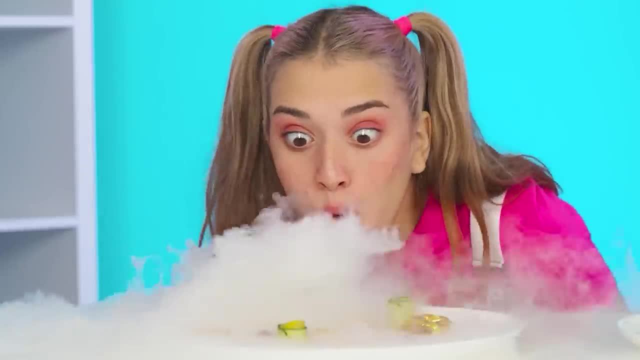 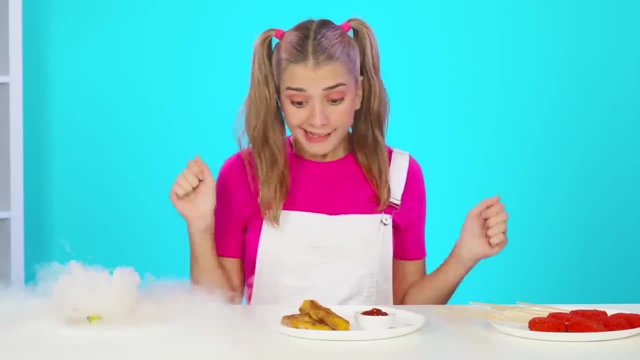 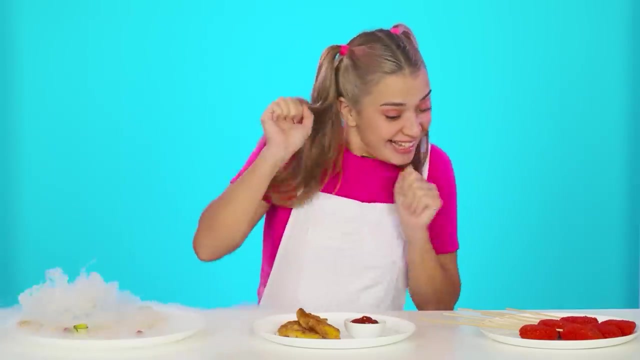 Oh my gosh, How cool it looks, Are these golden nuggets? They taste the most ordinary. Okay, I'll try the next one. Yes, I like these ones much more, But there are still some left Red ones- Great. 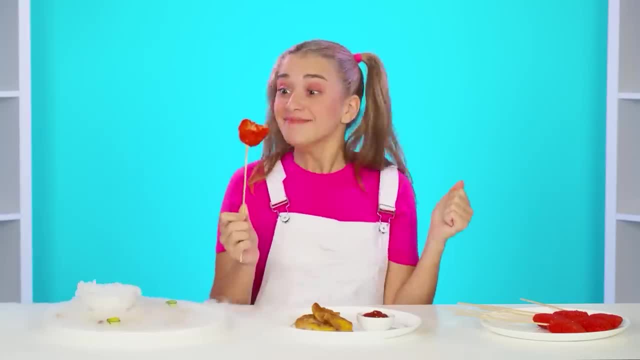 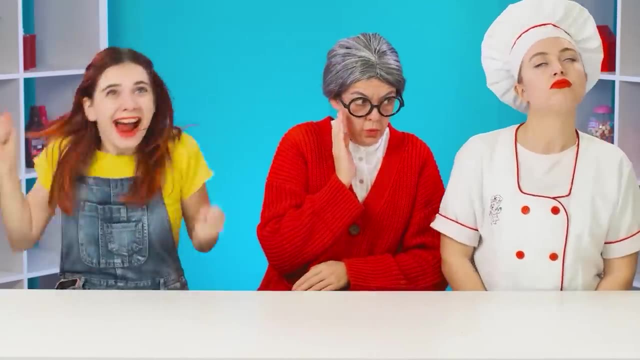 Mmm, There's Cheetos here too. This is definitely the winner. I'm one. Have you seen it? Have you seen it? Victory, Can you make pizza? I want it, No problem, I wouldn't mind it myself. 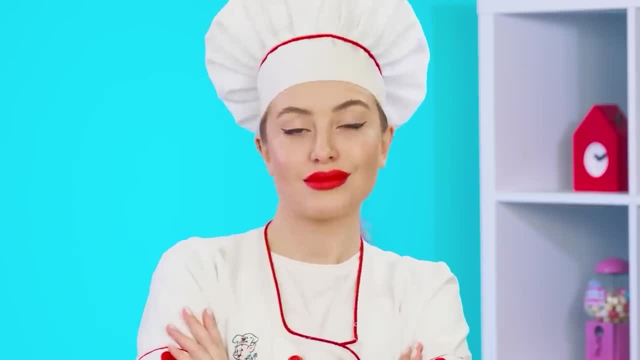 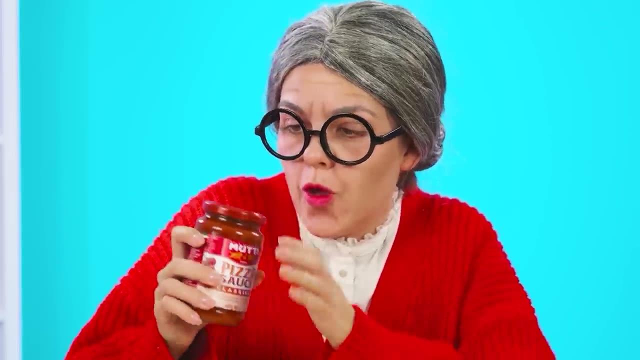 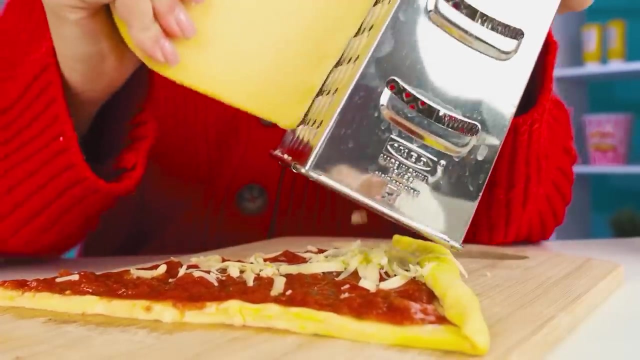 Ah, pizza, I can do that. Tomato paste is needed here. We drip a little on a piece and gently smear it with a spoon. And now the cheese. The more cheese, the tastier And pepperoni. I don't want it to strike bud. Look, I'm a chef Flying Dow. Look at this. A real increase in taste. This is so good, I love it. Oh my gosh, This is so good. It tastes better than the other kind. It's really delicious. 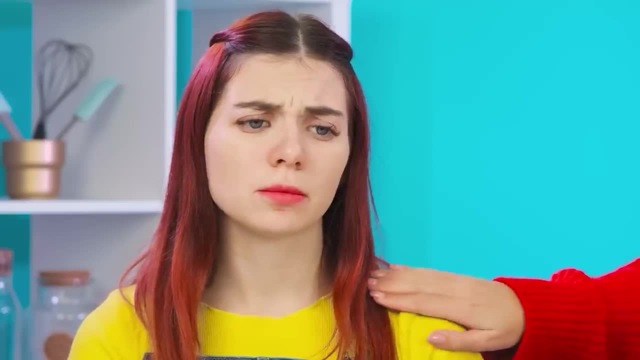 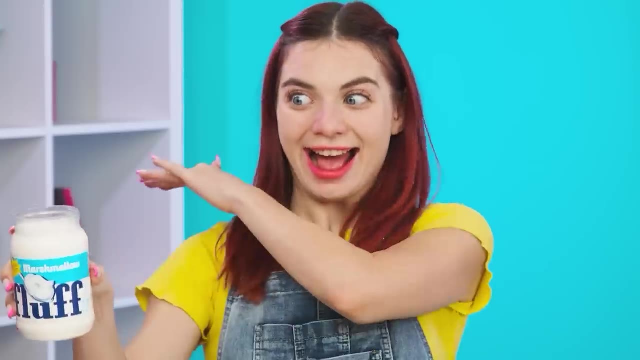 Oh, it did fly. Don't be upset, dear. Here, take a new piece. Thanks, Grandma. Oh, I know No boring tomato paste, But a marshmallow paste. I'll scoop up a whole spoonful like that. 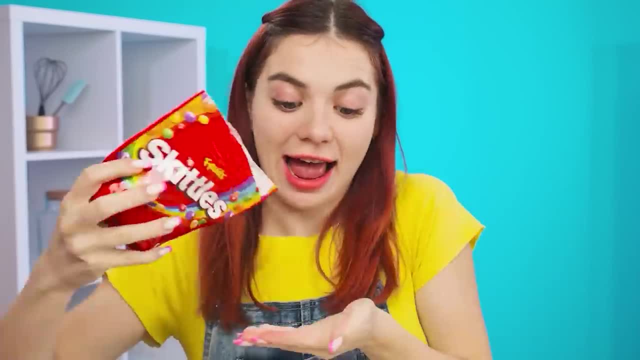 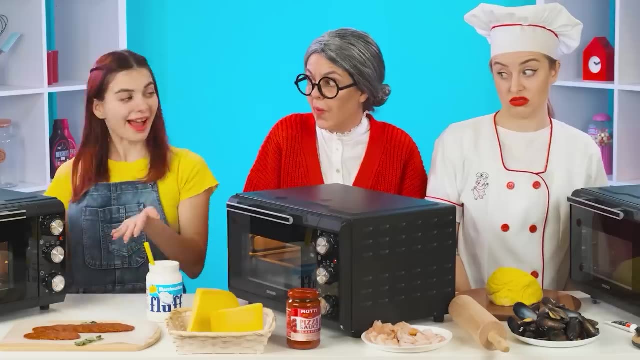 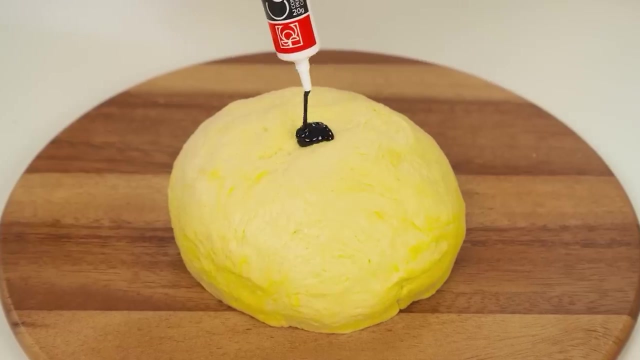 And now on to pizza And, of course, Skittles. They're never extra Well, I'm almost done. Yes, you can immediately see the hand of non-professionals. My pizza will be the healthiest. No boring white dough. 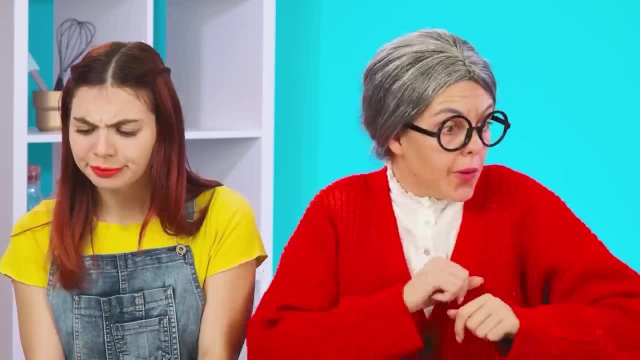 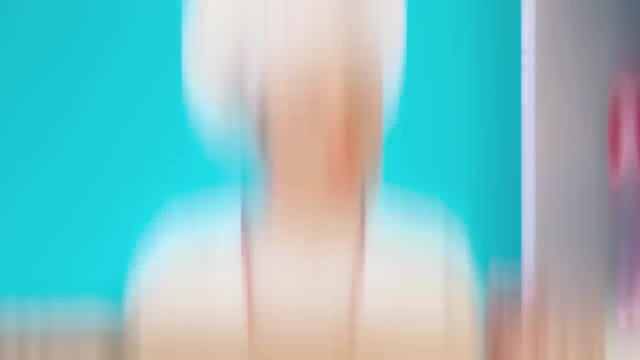 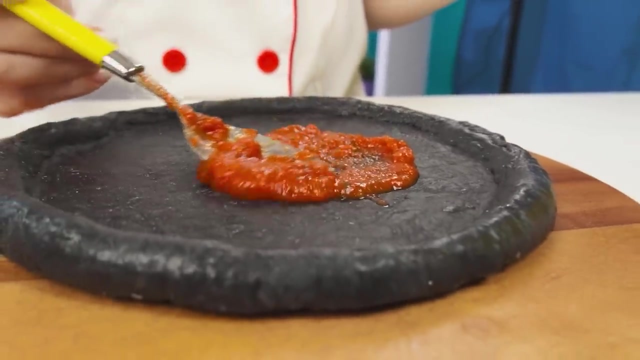 I'll make it more spectacular by painting it black. Oh, just look at that, I can do more than that. And now we roll out the base. The base should be smeared with a special tomato sauce. Then the pizza will be as delicious as in the best Italian restaurants. 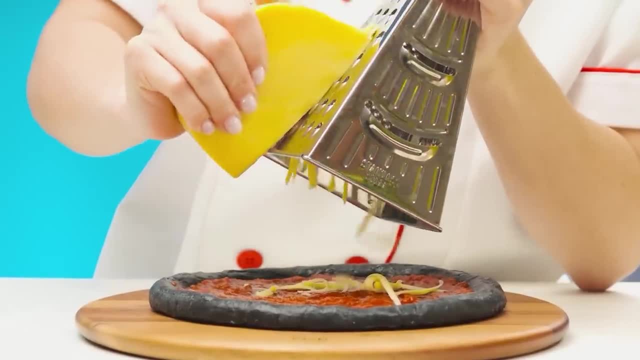 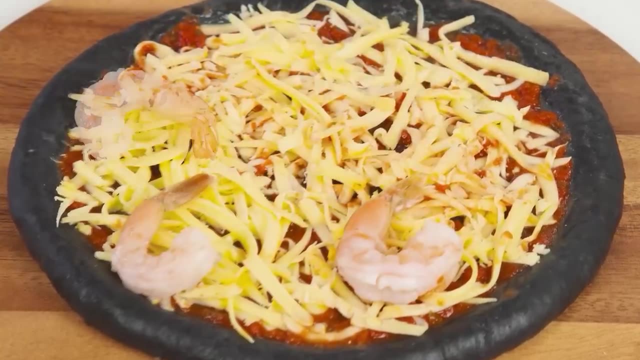 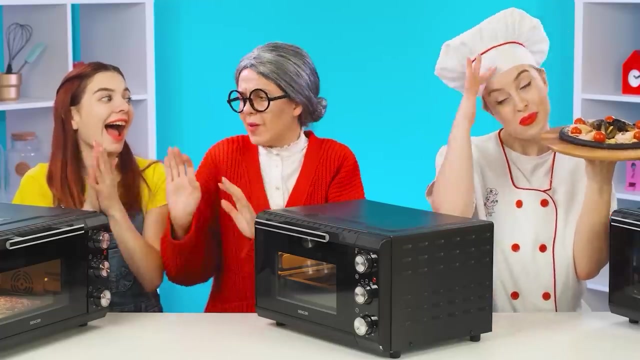 I'll put some cheese on top- Excellent. And now it's shrimp time, And so that they're not alone, I'll add mussel girlfriends. The high-cuisine dish is done. Get ready to enjoy. Oh, how long it's gonna take. 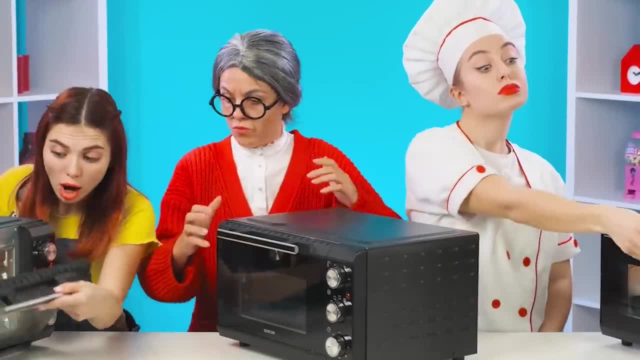 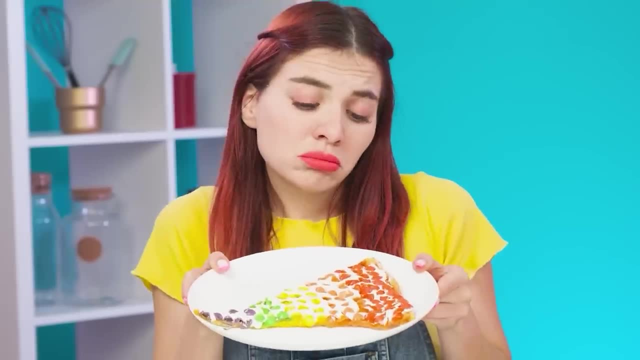 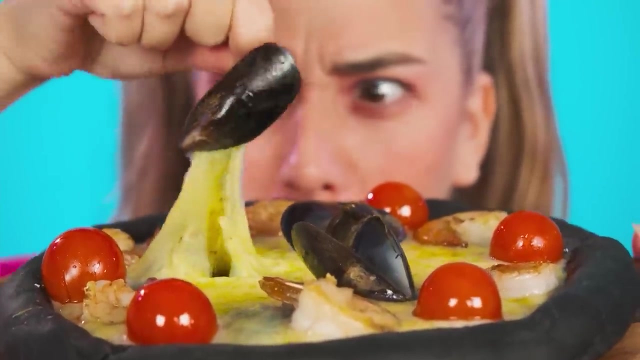 Oh, I think it's done, Perfect, Let's try the pizzas. Bellissimo, Yummy, Oh, so good. Oh, quite good, We'll see. we'll see How interesting it looks. What is that? Oh, are those real mussels? 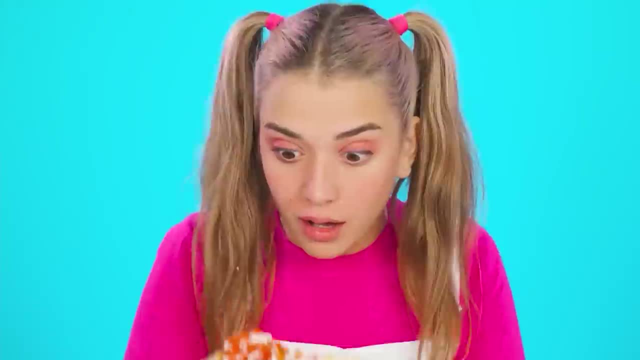 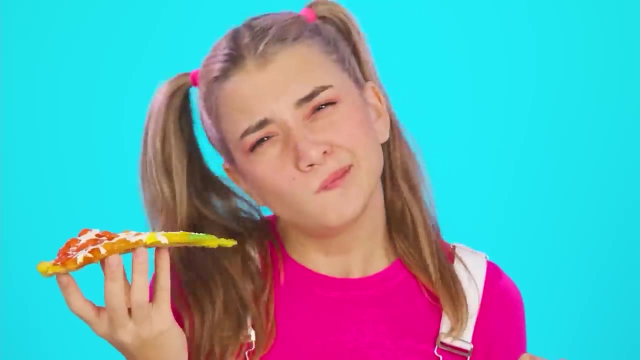 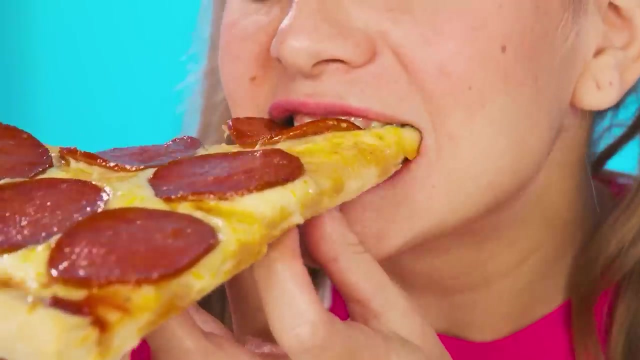 I'm not gonna try it, But this is more interesting. Looks like Skittles. Um, it looks better than it tastes. Oh, but this pizza looks completely normal And it smells so good. Mmm, what an amazing taste. 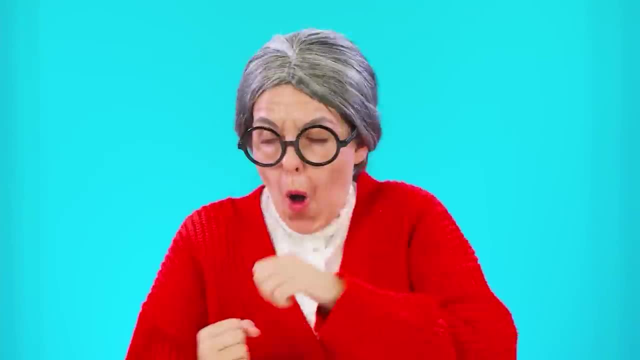 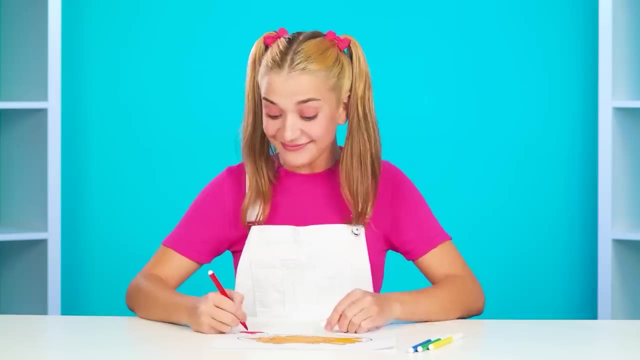 Yes, it's the winner. Congratulations grandma. Oh, a well-deserved victory. My pizza was better, No comments. So the heroes have a responsible task to feed the baby. And what does she want? The baby wants french fries. 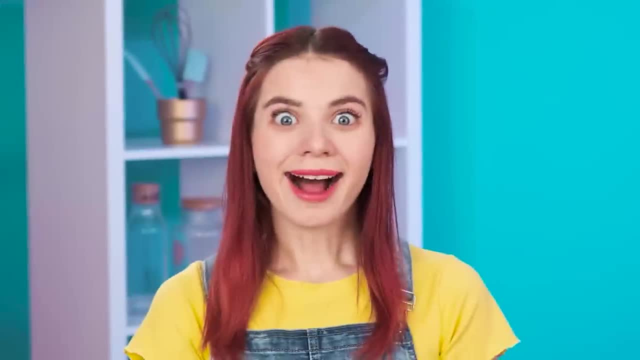 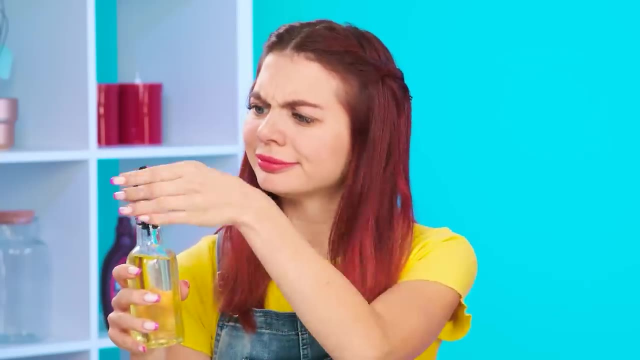 Nothing complicated. We'll do everything. I know the recipe. It seems that you need to pour oil. I'll pour more. It'll be fatter and tastier, So for sure everything will fry. well, I'll fill up the whole pan with some oil. 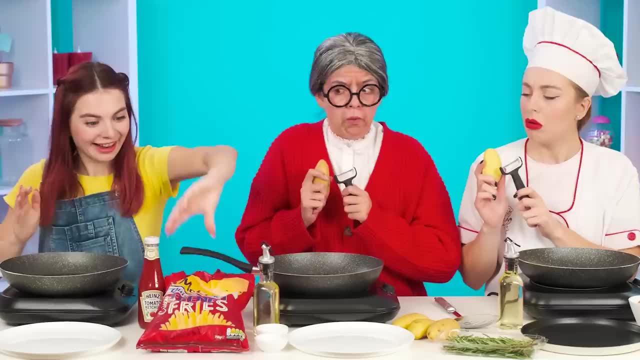 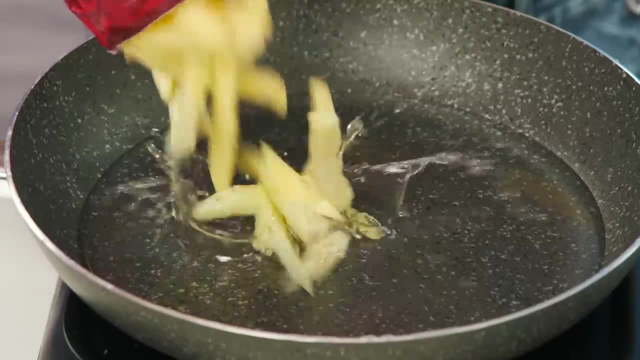 Let's turn it on And let's start. I'll use the whole pack, because there are never too many of the french fries. Granddaughter, what are you doing? Oh, it's burning. We need to put out the fire quickly. 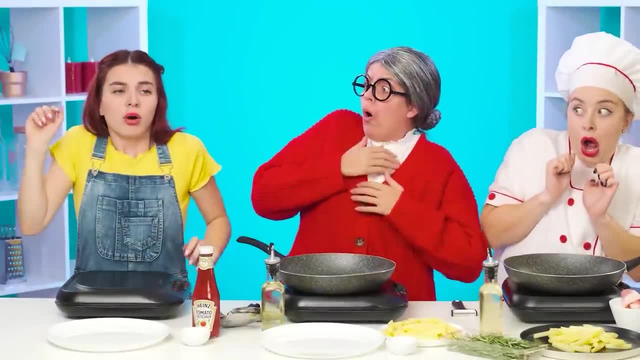 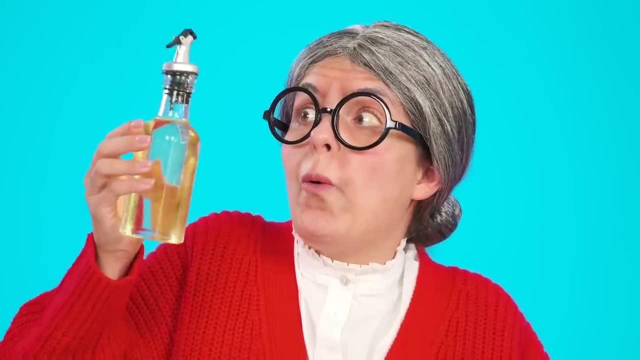 Oh no, no, It's not like the recipe on YouTube. Almost burned down the kitchen and all of us Better learn from grandma. Now grandma will show you how to do it. We'll take quite a bit of oil. Turn down the heat a little. 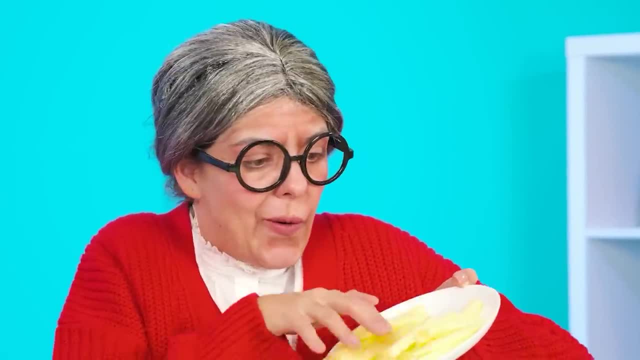 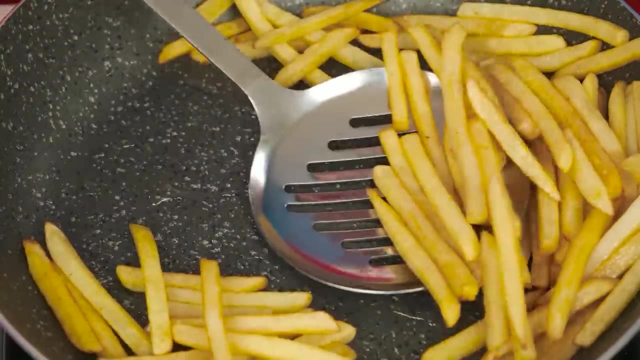 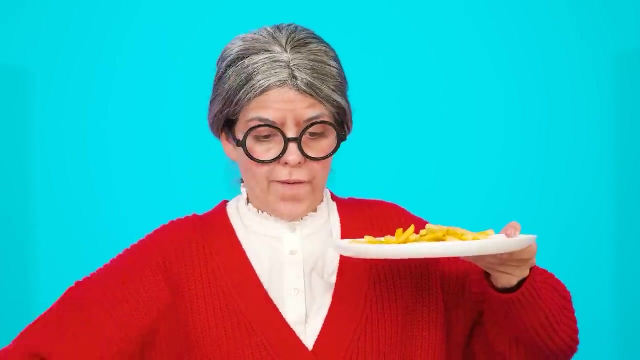 And put the potatoes in. So it'll be perfect. I'll toss it around And put it on a plate. What, Oh, how well it turned out. It's going to be perfect. It's going to be perfect. It's all for my granddaughter. 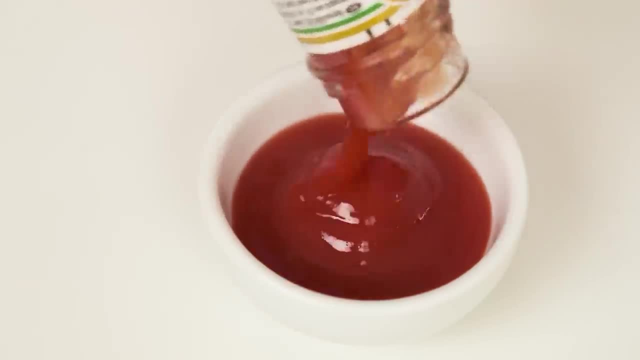 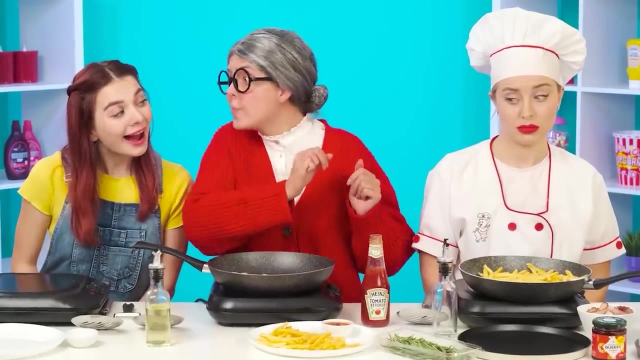 It remains to add the most delicious ketchup. It remains to add the most delicious ketchup. French fries and ketchup are the perfect combination. French fries and ketchup are the perfect combination. My granddaughter will definitely like it. My granddaughter will definitely like it. 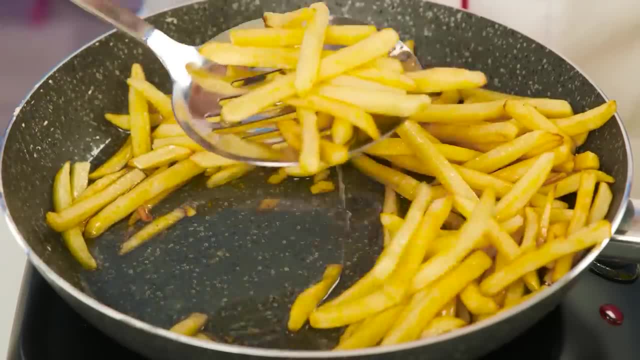 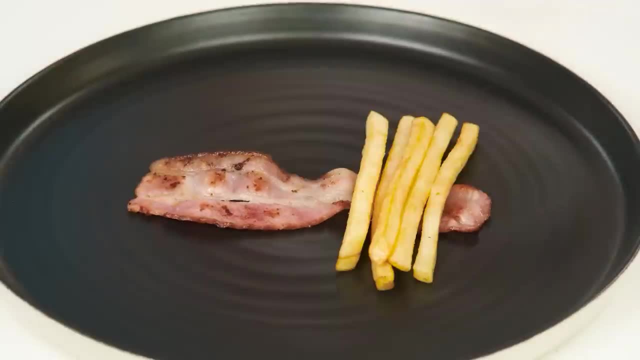 And how many calories are in this dish. I'll show you how it should be. We get rid of excess oil, Then we wrap the potatoes in a piece of fragrant bacon. Then we wrap the potatoes in a piece of fragrant bacon and twist the roll. 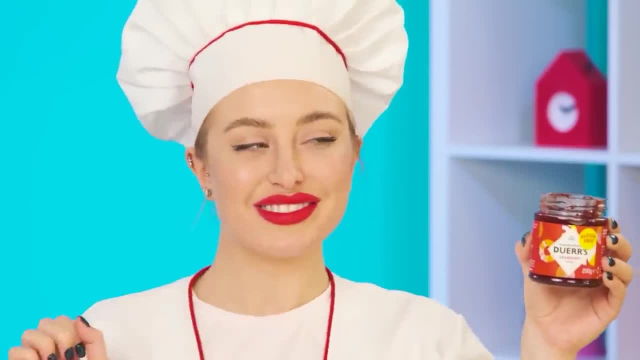 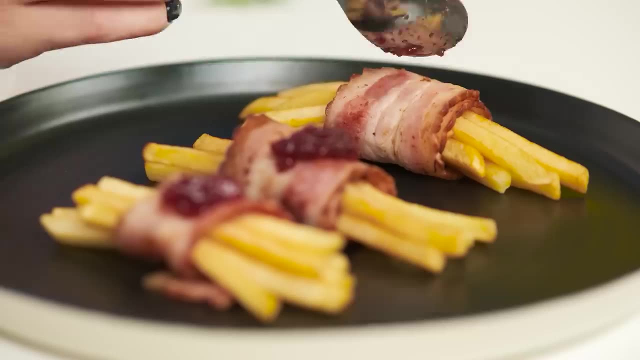 Just like that. Add a drop of cranberry gluten-free jam. Add a drop of cranberry gluten-free jam from Duro's on top- from Duro's on top, Just like that. And add some rosemary on top. The masterpiece is ready. 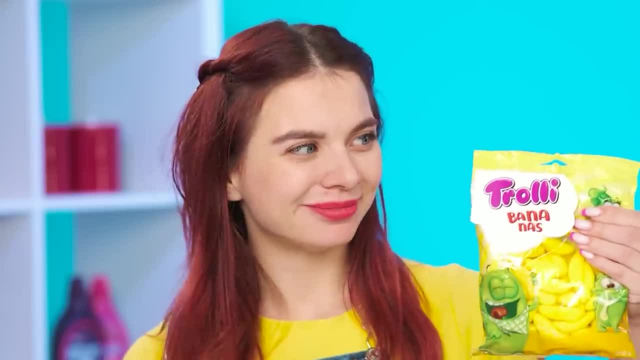 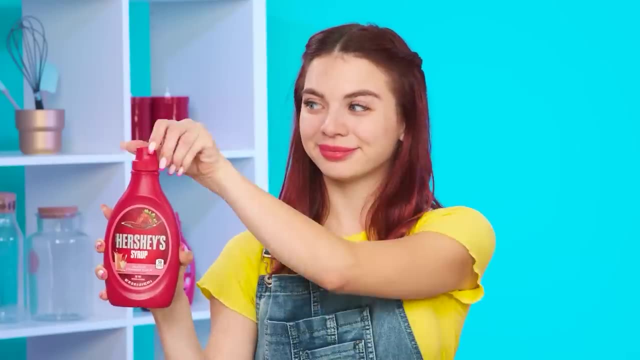 The masterpiece is ready. I've come up with something better: Banana marshmallow. choli is so similar to potatoes And if you add Hershey's strawberry syrup it'll be just like potatoes with ketchup. it'll be just like potatoes with ketchup. 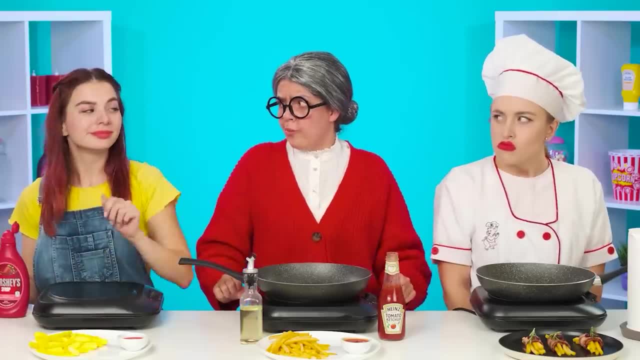 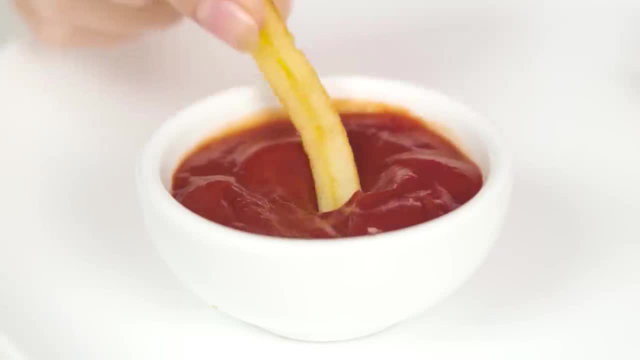 It's so sweet. That's what my little sister will really like. That's what my little sister will really like. Finally, everything is ready And the baby has already been waiting for her food. The dish from my grandmother was the first to attract attention. 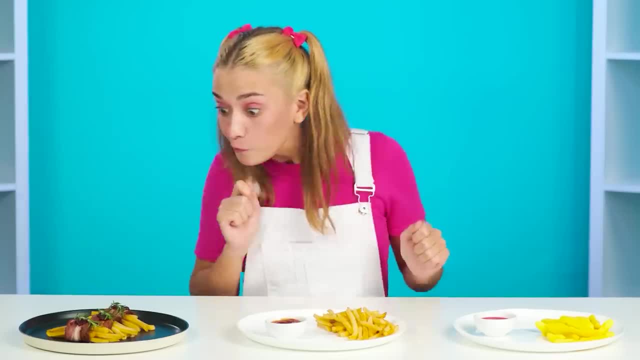 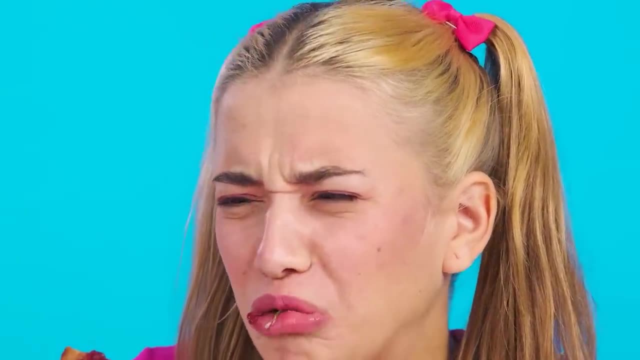 Classic french fries and ketchup. It looks really delicious. The baby obviously liked it. I wonder how she would like a dish for real gourmets. The chef took an unusual recipe, but it was not appreciated And there was a gift. 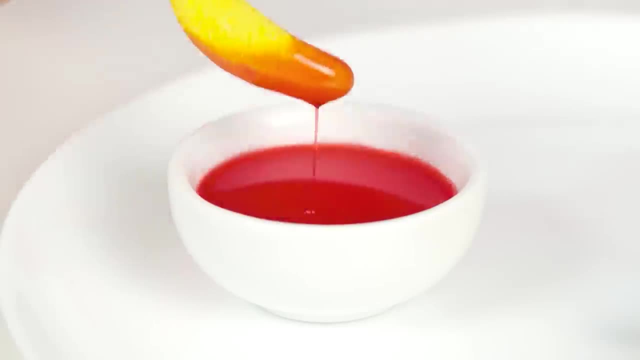 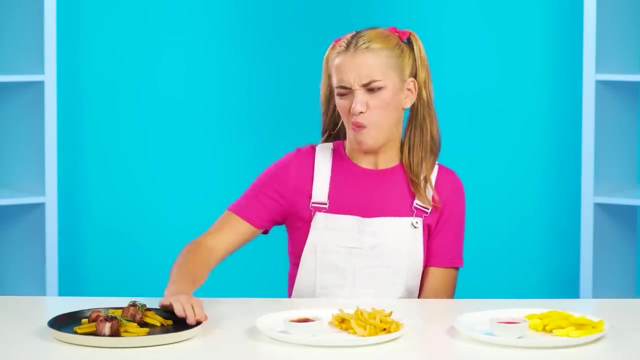 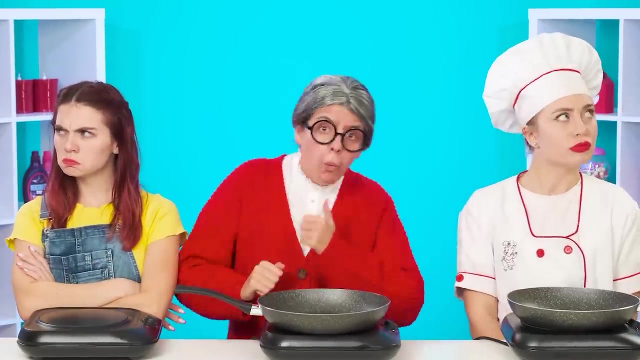 from my sister. It looks like potatoes and ketchup, but this… Yes, It's a sweet marshmallow with strawberry sauce Deep and eat. It remains to choose the winner: A dish from grandma? Yes, I won. Oh, It hurts. 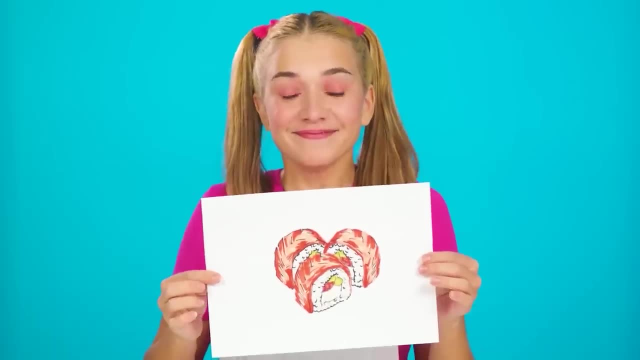 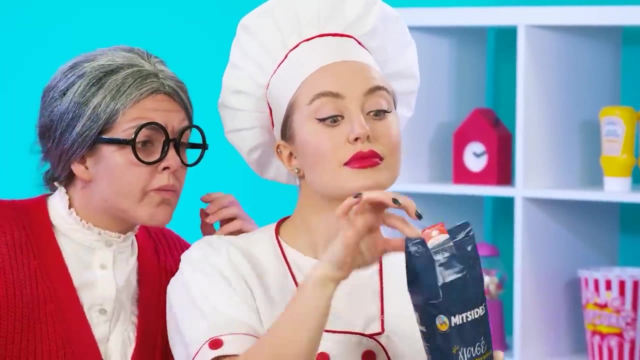 What will the baby want to eat now? Oh, she wants to eat sushi. Oh, she wants to eat sushi. What is this? Do you know how to cook it? Show grandma what to do. First, you need to boil the rice in a special way. 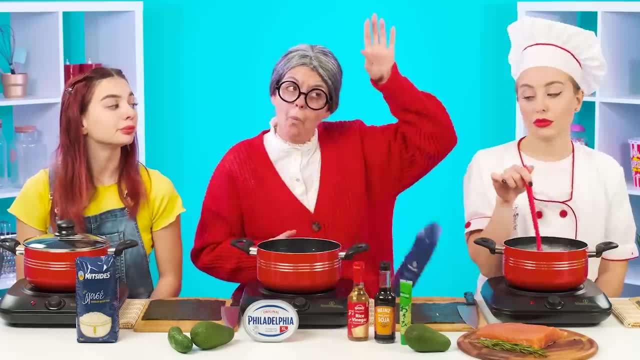 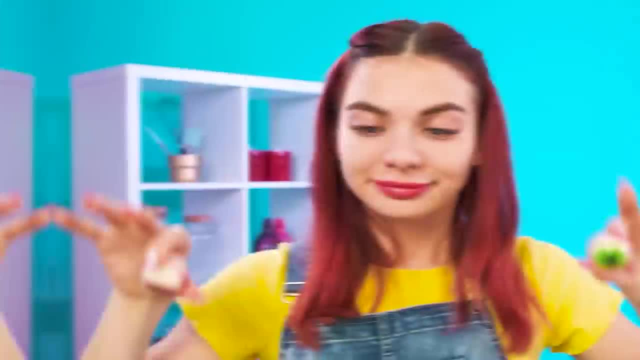 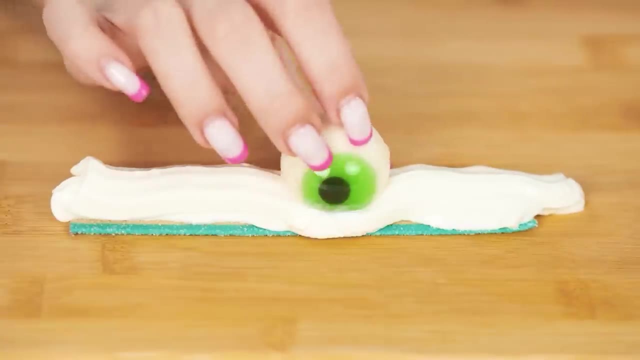 I'll do it. Grandma knows how to cook rice. Ah, Sushi with nasty seaweed. I'd rather do something sweet again, Or sweet and sour. Let's take the sweet and sour tongues. Add whipped cream instead of sauce, Wrap a marmalade eye. 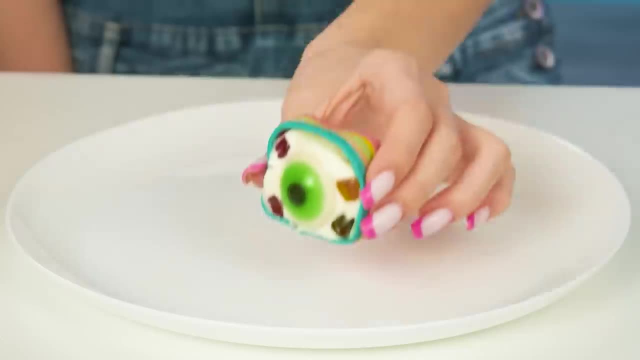 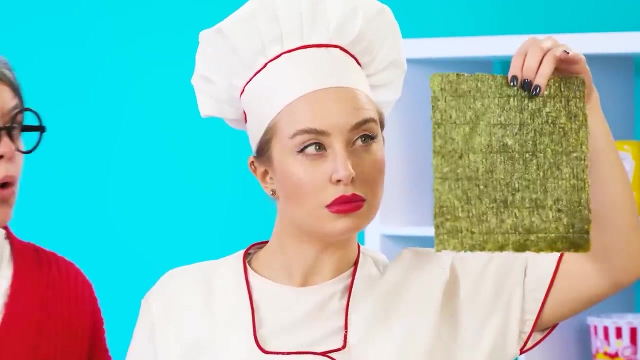 and a few marmalades from Haribo. How big and colorful they turn out. Have you ever seen sushi like that? This is just absolutely perfect. Now you need to take a sheet of nori and cut it in half. It's all dry. 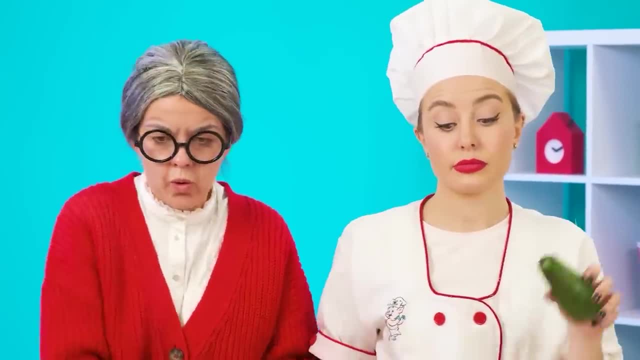 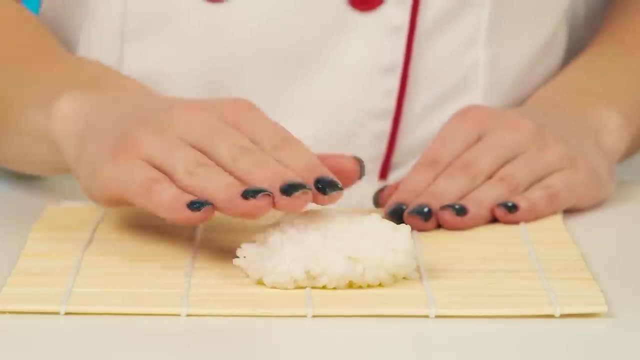 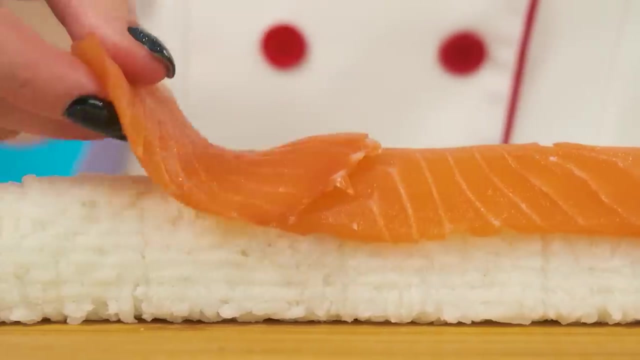 It's breaking. How did you do that? Because I'm a professional grandma. I'm gonna cut some fish, Perfect slices. Put some rice on the mat and some nori. I twist it with the mat, Put some fish on top. 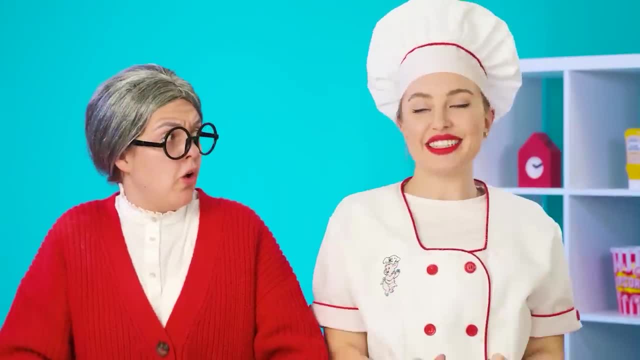 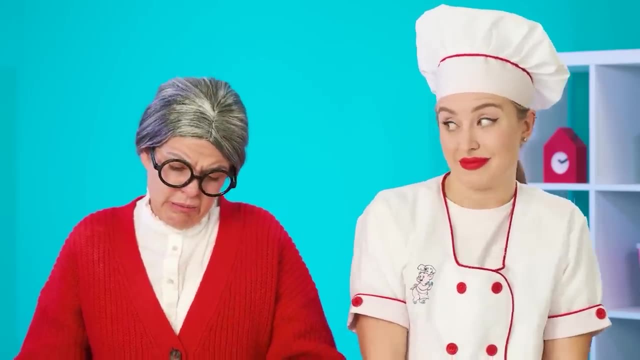 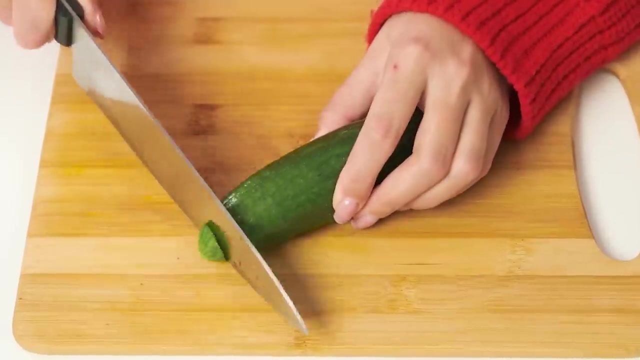 Cut it And that's it. Classic Philadelphia roll with ginger and wasabi is ready. Granny can't make these rolls of yours. They don't keep their shape. Bingo, I have an idea. I'm just gonna cut some cucumbers. 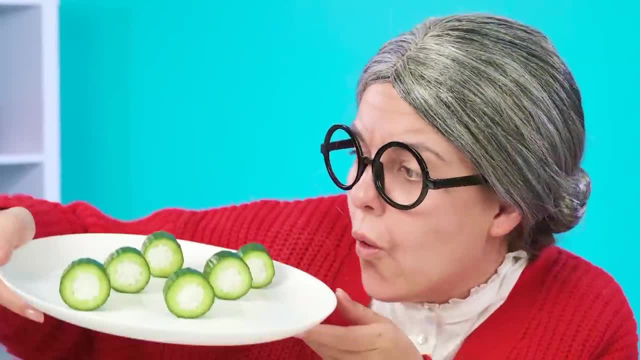 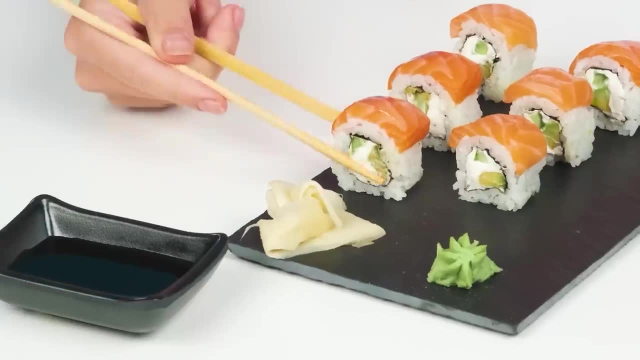 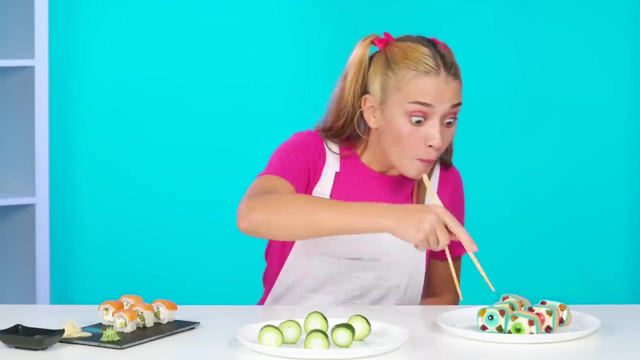 Get rid of the center and put rice in. Perfect. Now it's time for the baby to try it. Let's start with these Sushi from the chef. looked perfect And it tastes incredible. What a big and bright roll And very, very tasty. 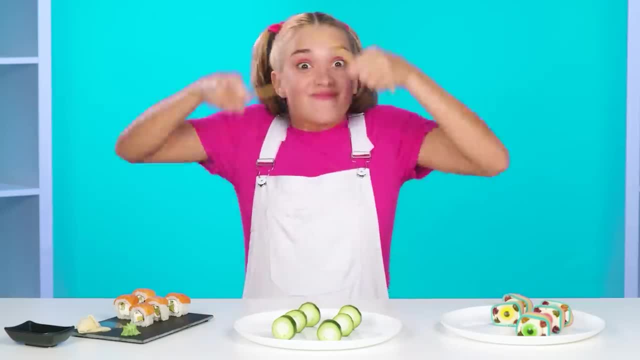 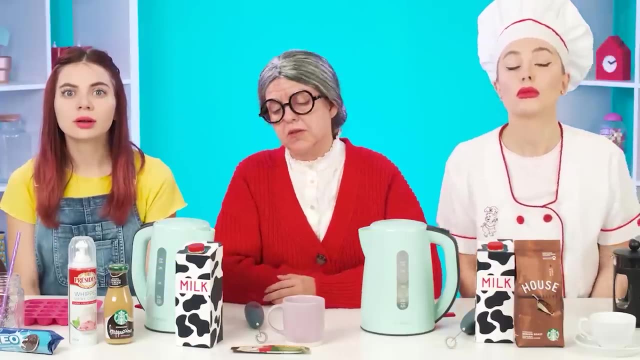 So delicious that she immediately chose them as the winner. This time, a sweet gift from my sister overcame everyone. Oh, you haven't tried mine. Hey, grandma, wake up. My daughter wants something delicious again. She wants to drink a chocolate cocktail. 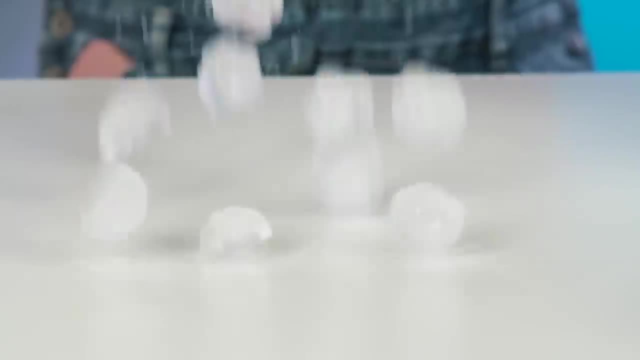 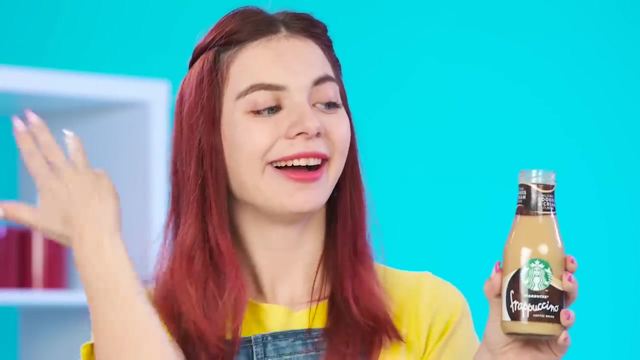 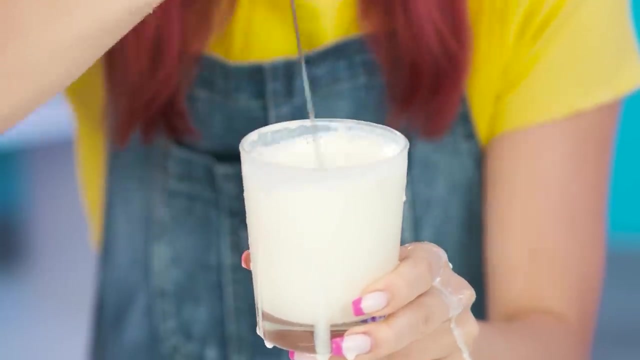 for dessert. This is my favorite recipe. We'll need some ice cubes. I'll pour more chocolate sauce into the jar- Starbucks milk chocolate to the brim And I'll create some milk foam with a hand mixer. Oh, um, sorry, grandma. 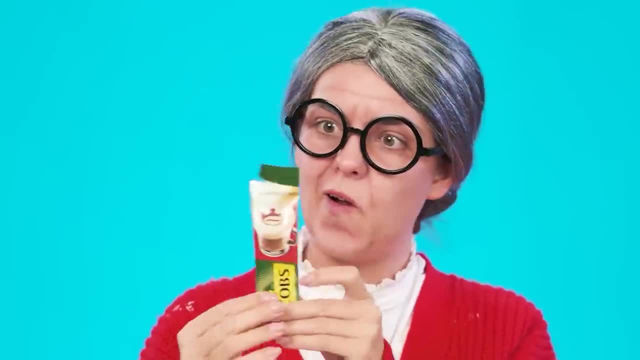 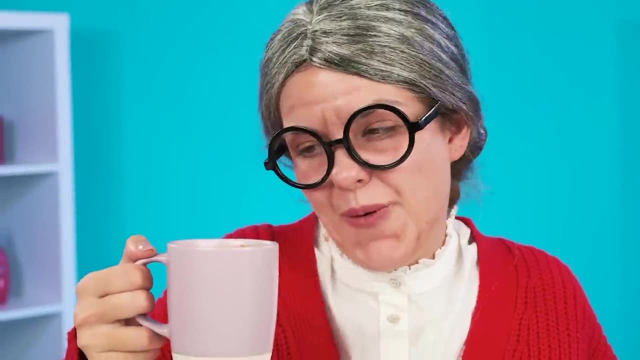 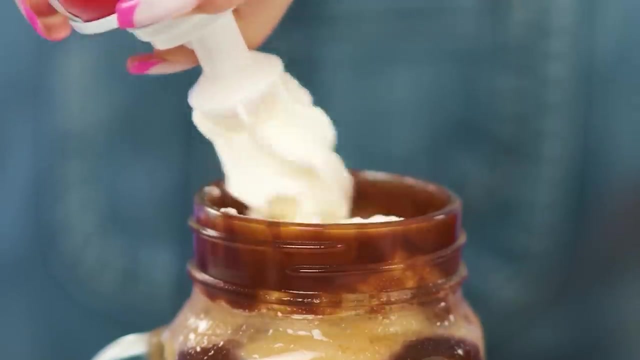 You got too close. What is this bag in grandma's hands? Instant coffee 3 in 1?. Is she really going to give this to her granddaughter? Yeah, but it seems that grandma herself likes it. Now add the whipped cream. I often cook myself such a recipe. 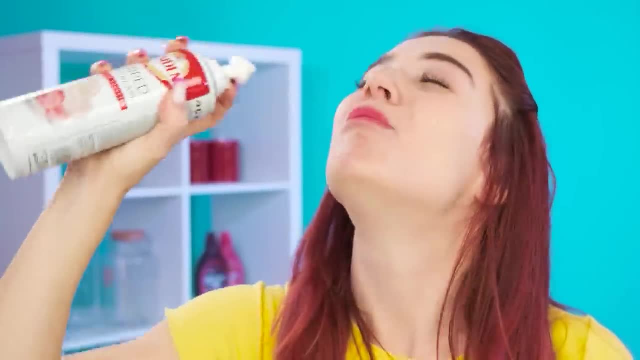 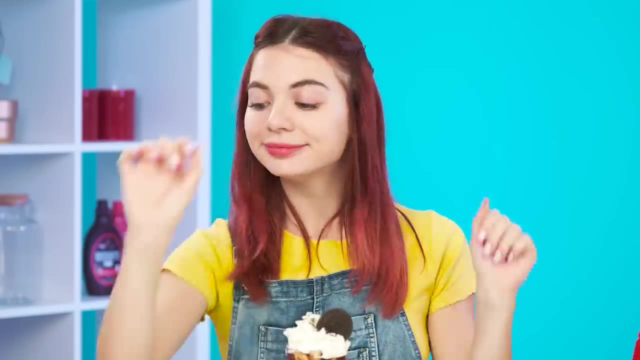 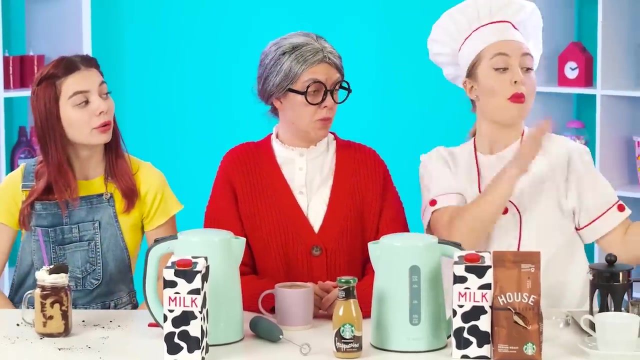 By the way, don't forget about yourself. Sprinkle the Oreo cookie crumbs on top. Put the cookie on. Such a cocktail should be drunk through a straw. That's it, The perfect chocolate milkshake. Who cooks it like that? 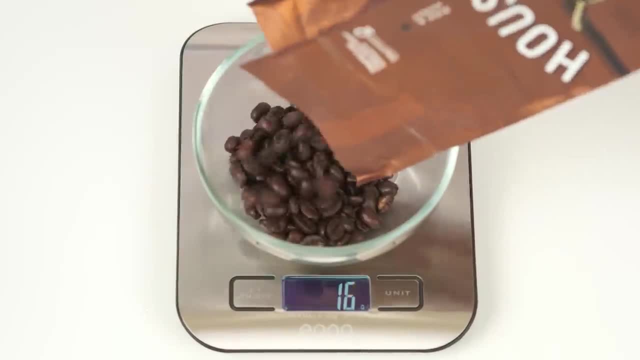 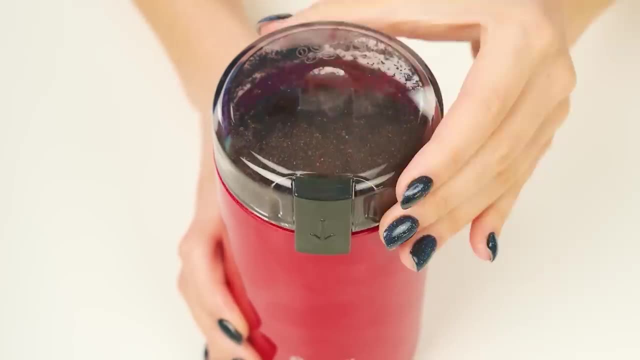 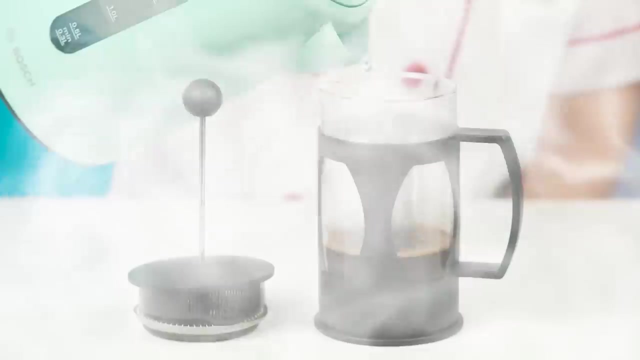 That's a horror. I have made coffee sweet drinks more than once. We need fresh coffee beans. I measure everything to the gram. I grind the grains into fine crumbs, Then I brew it in French press. The coffee will be perfect. Pour it into. 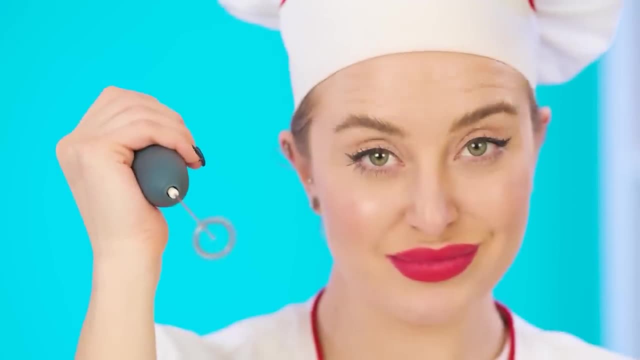 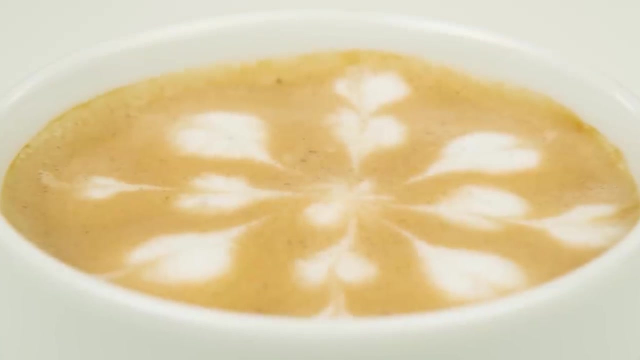 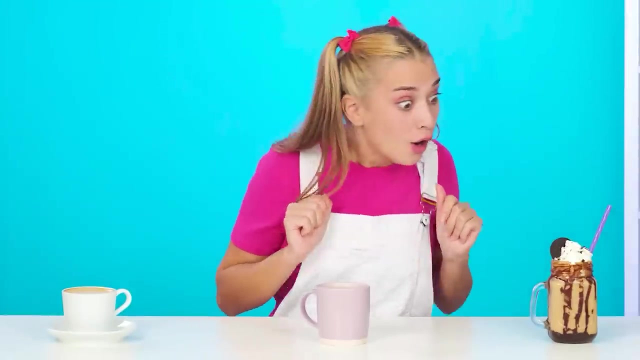 the cup And adding some milk. I'm going to create some foam out of it. I certainly won't spray anyone, because I'm a professional, And the snowflake decoration- Perfect. Oh my, It's time to try the drinks. The hand itself reaches for beautiful glass. 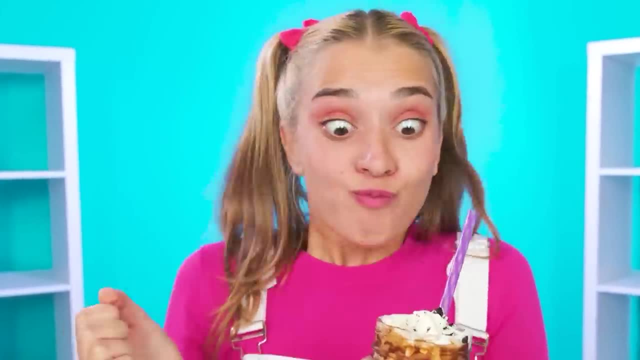 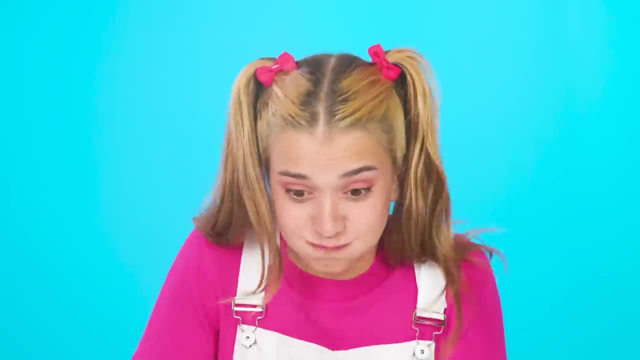 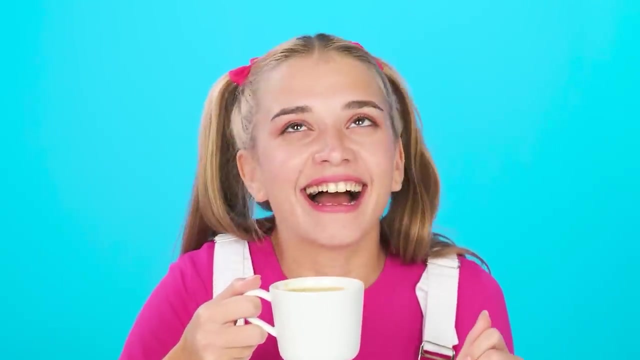 It's a wonderful cocktail. Also, delicious cookies on top. It's perfect. What can not be said about the instant coffee? Grandma wanted to poison her granddaughter. It's impossible to drink Coffee foam from the chef with a pleasant aroma, But the taste. 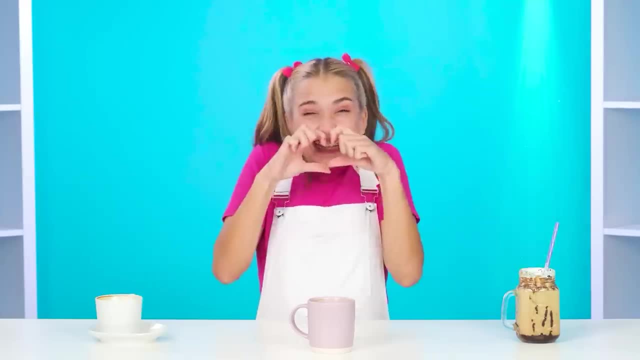 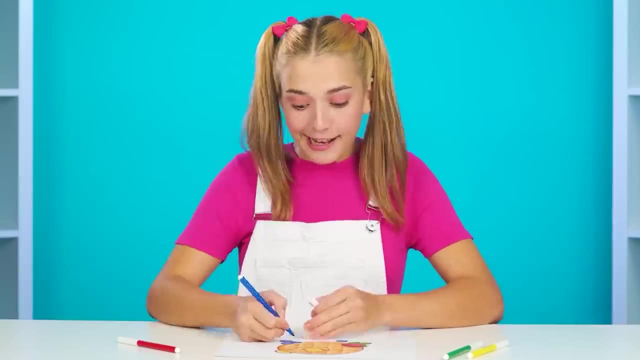 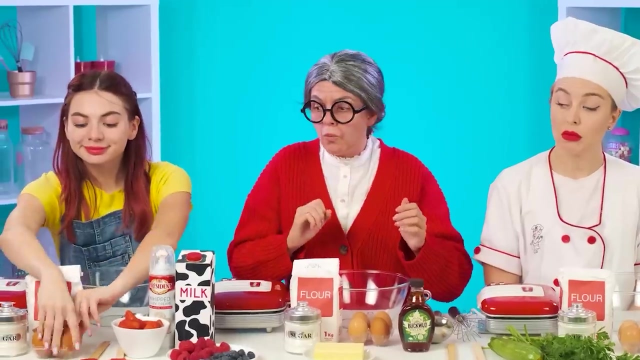 is nothing unusual. The baby chooses the beautiful cocktail. Yes, keep it up, sis, You've won again. The next task is for you to drumroll. make some waffles. Okay, What, What is it? And I know the recipe. 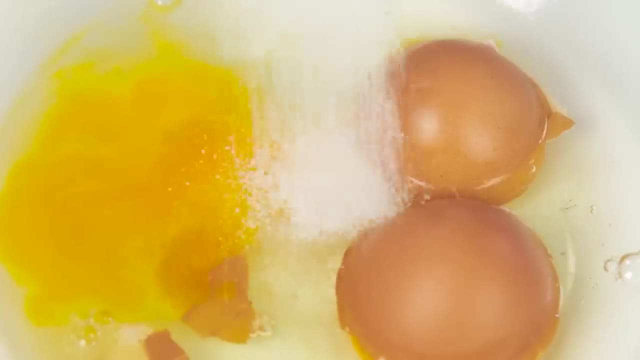 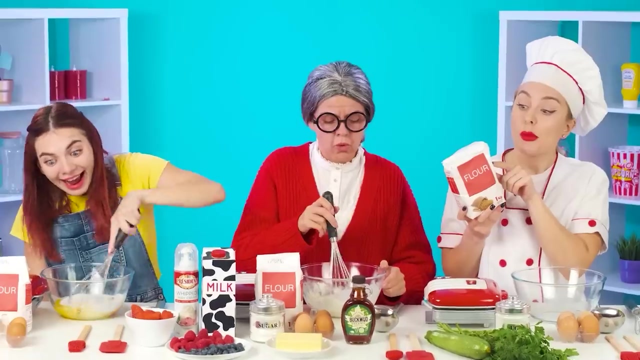 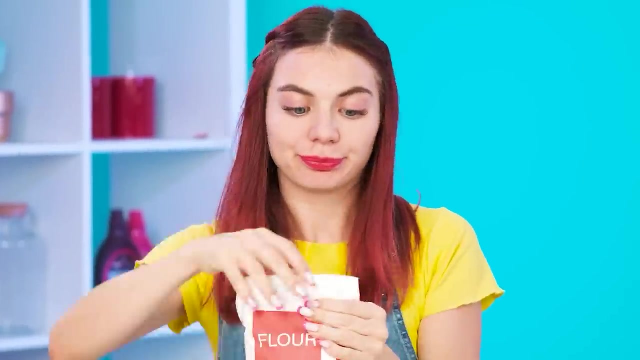 Break the eggs, Add sugar- You can have more, so the waffles will taste even better- And get in the way. get in the way, get in the way. Oh, I'm tired of doing that. Perhaps that's enough, And now we can add some flour. 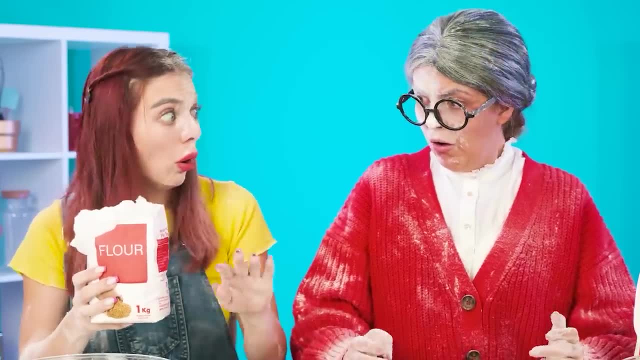 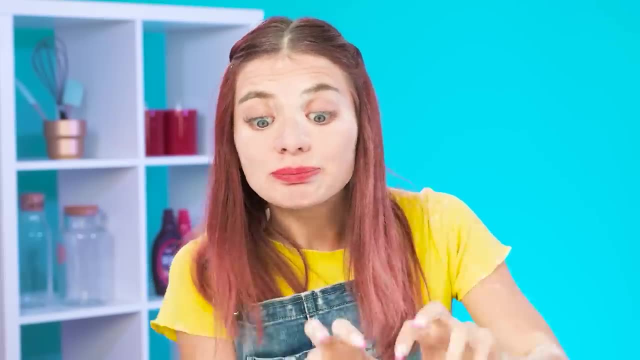 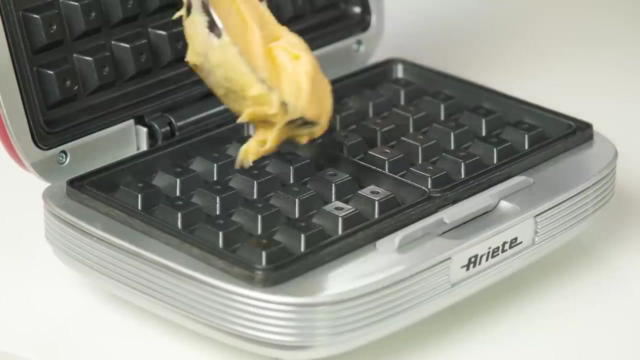 How much is needed? Oh, Grandma, I'm sorry, I got you dirty Again. More flour, more waffles? Uh, maybe you don't eat so much flour. I'll put the excess back. It won't work out that way.